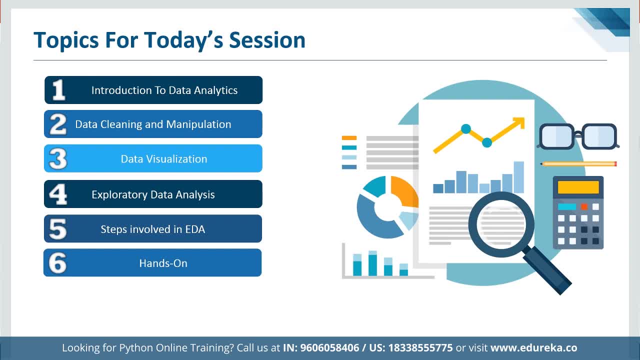 talk about exploratory data analysis. Okay, So you all know that today's agenda basically will go: what is analytics? and then we'll go into the major steps in this artificial intelligence and machine learning, which is EDA, and we'll talk about that EDA extensively and then we'll look into 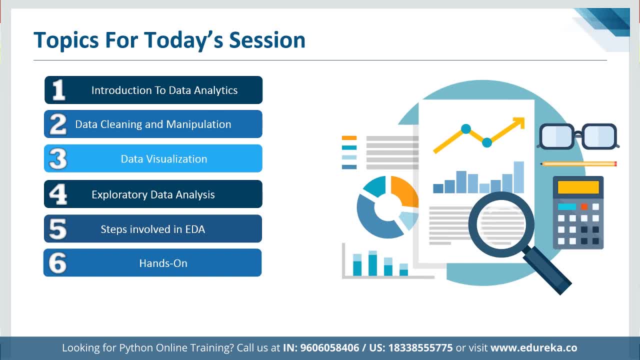 basic one case study. Okay, that in python will go over that. Okay. so these are the topics for today's session: Introduction to data analytics, data cleaning and manipulation, data visualization, exploratory data analysis and the steps involved in EDA and heads on Okay. 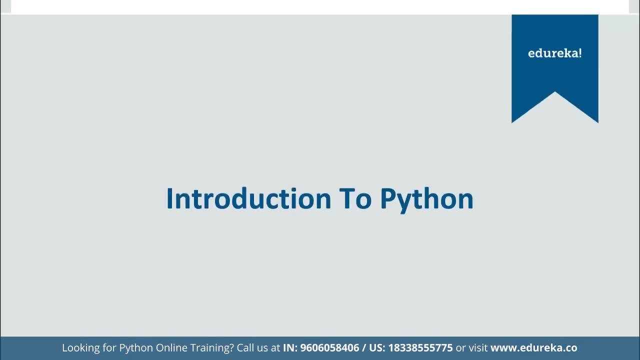 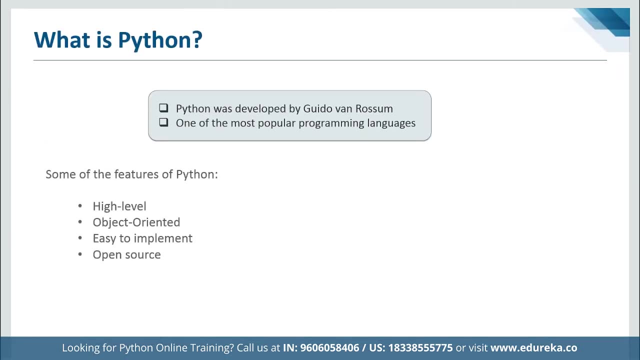 so let's see what is python, Okay. so basically you all have a basic idea about artificial intelligence, right? So artificial intelligence basically is a field which is all the things are happening now, and machine learning and deep learning, NLP, all these are in that field, basically artificial intelligence, areas of that field. these are So to implement. 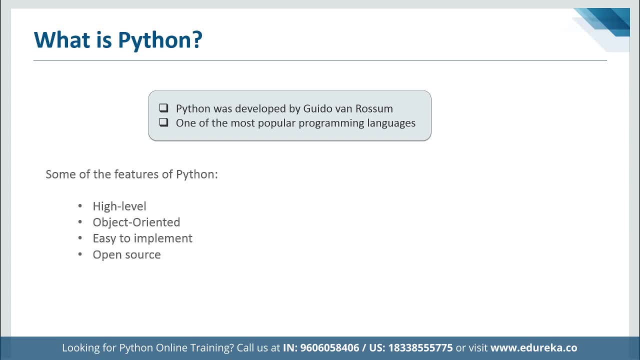 this one. we need a programming language. Okay, there are few programming languages that we can use here. We can use java, we can use python, we can use julia, we can use r- Okay, but in the last two, three years, python became the de facto industry standard for artificial intelligence. 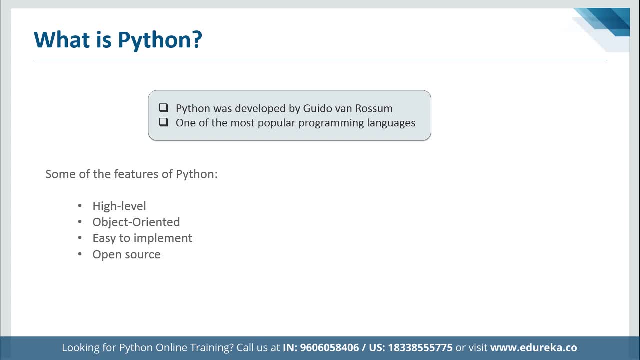 Most of the companies are using python now. That is the reason that it became the most popular programming language last year. How do we know that it is the most programming language? Because the number of projects, number of people working and number of questions asked in 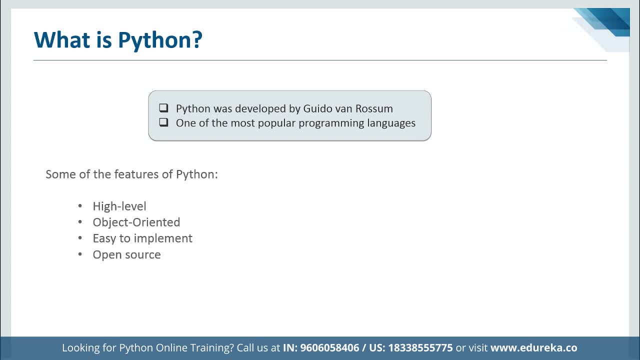 stack exchange and all those forums. Those are kind of metrics that we use to see that which is most popular language. So this is not a new language. It was developed by Gideon long back- about 20 years back, Okay- but it came into prominence recently after the emergence of 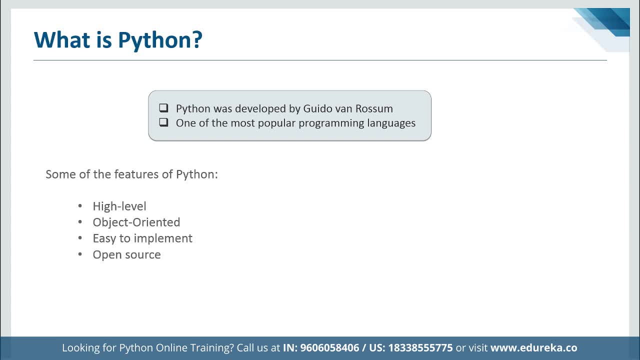 machine learning and deep learning. Okay, so it is a high level language. That means basically you just like english, like coding. Okay, you can easily understand even a person who doesn't know anything about computers. They read code, They know that it is what basically it is doing It. 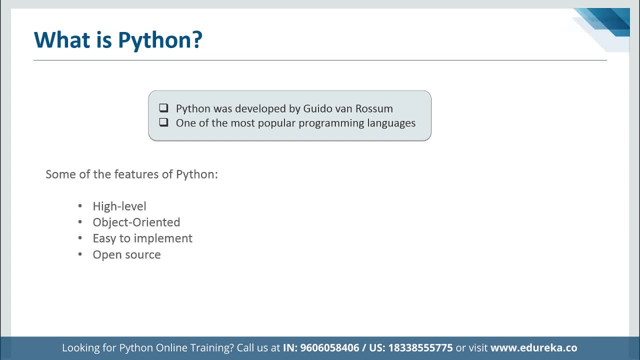 is kind of high level, not at the low level like compiler or something like that. So it is a high level language in terms of code. Okay, it is object oriented, So basically you can take advantage of its object oriented concepts and programming aspects of it So the code can be clean and 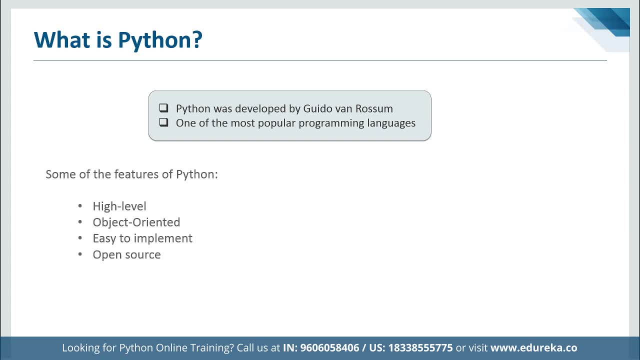 modularized code. Okay, and it is easy to learn, easy to implement. Basically, I learned about 10-12 languages in this last 20 years and this is easiest language and many people work for that. Okay, and most important, it is open source. that means that you don't need to pay anything, you just download and you can use it. 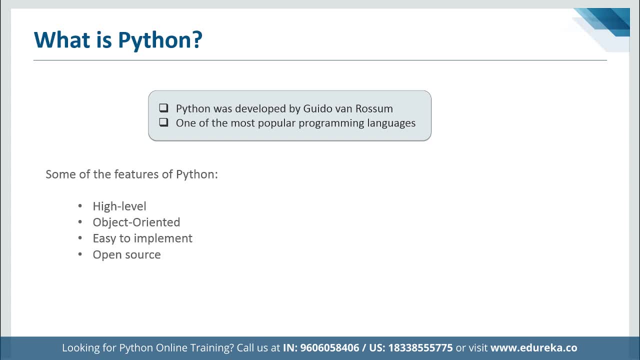 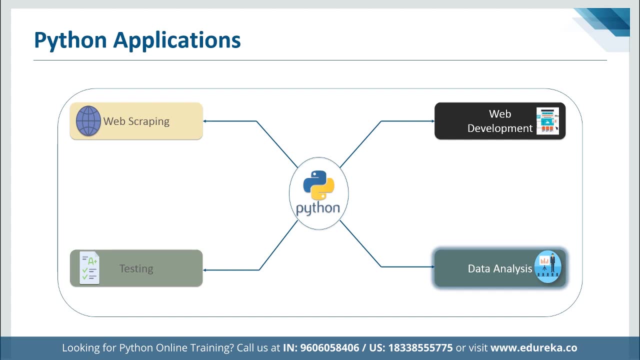 okay, that is about python. python can be used for lot other things other than artificial integers. basically, you can build websites. you can do a lot of things. you can do web scraping. that means you want to get data from the web. suppose, like drug research, data from 10 pharma companies, you can. 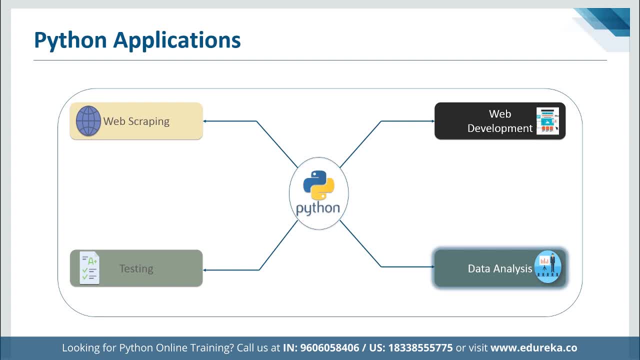 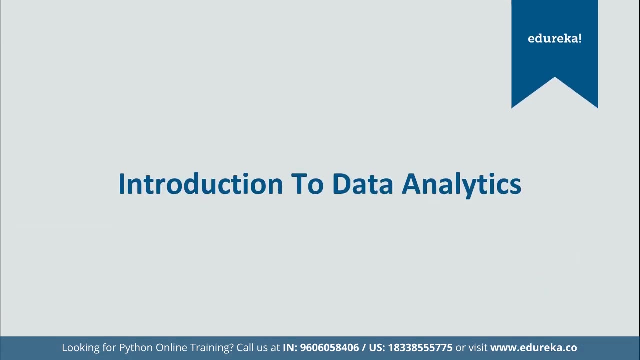 do web scraping and get all the data- okay, and you can do a lot of things with python, but here we look at what the aspect is with artificial intelligence. okay, so let us look at what is data analytics and why data analytics- basically data analytics for any corporation or for any. 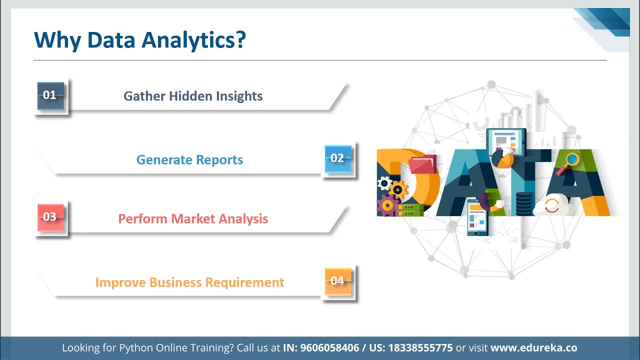 government or non-government organizations. data analytics gives the hidden insights into the huge amount of data data. now you saw that covet 19- we got a lot of insights into the spread and the death rates and morbidity. all the data that we got is from the analytics that we generated from the huge amount. 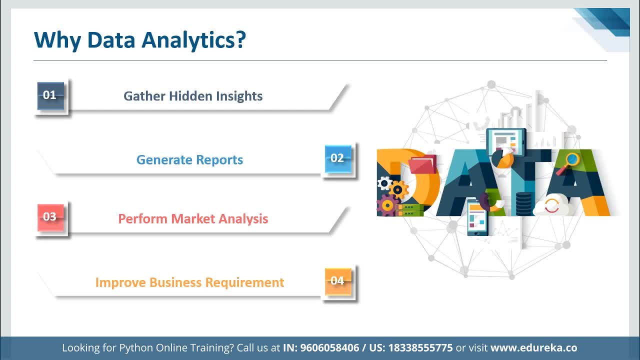 of data that all the world countries and who is so? data analytics is the graphs and all that you are seeing in the websites on the tv. basically, this is generated by the data analytics. so why it is important? because for common man or for a management, easy to see. 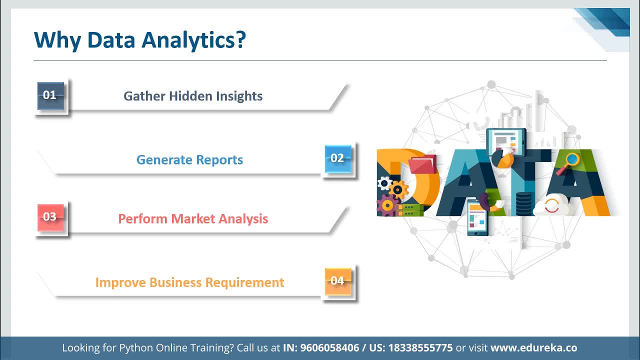 data analytics are gives a big picture of the huge amount of data. they may not have the time. even common population will not have time or energy to understand all the data. so basically this will take the important aspects inside and just put it in a graphical form. so for us, we know that okay. 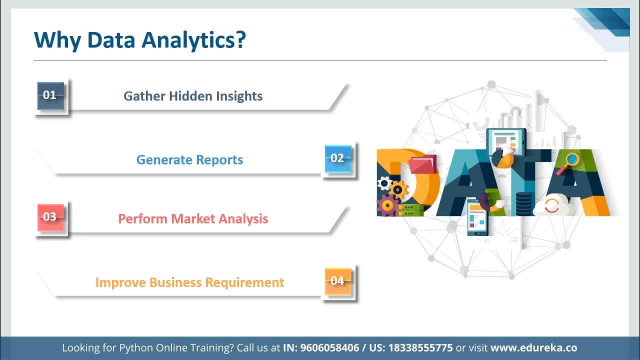 with this graph is: uh, the virus is uh, spreading like this one. it is flattening, or this is the ratio. how many people are getting this? all this kind of data that is useful for a population and for a corporate- maybe market analysis, or performance reports, or stock price analysis- all these things are sales, especially. 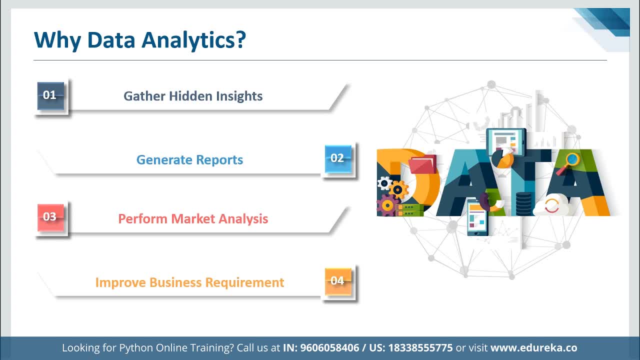 sales and all these things. you need that kind of information. the management need that kind of information. real time in the information. okay, to take decisions on where to spend their advantage money, what kind of products are popular in what kind of segments. all these things, which customers are leaving and what. 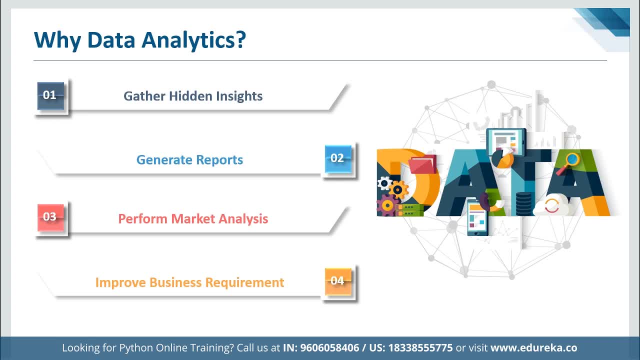 customers are finding it is good, what products are popular. there is millions of questions that management will have. this will answer all those questions. okay, so that is the reason of importance for data analytics. okay, so let us go to the next one. so what is data analytics? refer to the techniques. 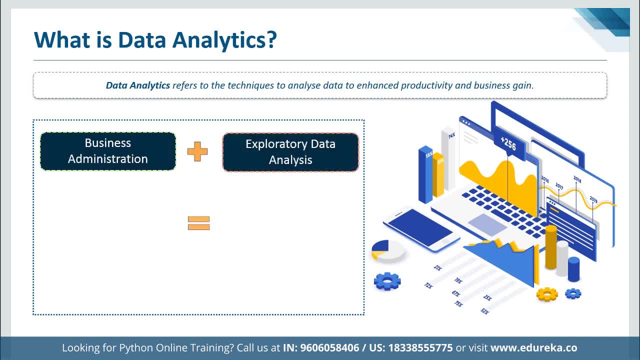 to analyze data to enhance productivity and business. so that's the reason that data analytics play a crucial role for the management. okay, so, basically, you have the business administration and the eta, you use it to get the insights into data and that will propel your growth business. okay, so who is a data analyst? basically, what are the roles for a data and this? basically, 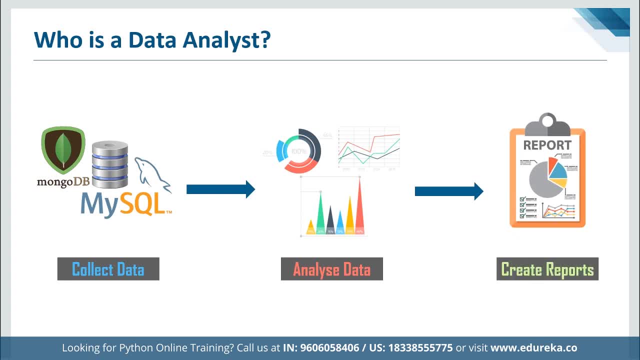 in the business world. you see that business analyst, data analyst, data scientist and data engineer- these are the common roles here. data analyst and business analyst are kind of beginner roles where they know about the data. they know sql, they know the relational database, how to access it and how to manage the data, how to manipulate the data. okay, so 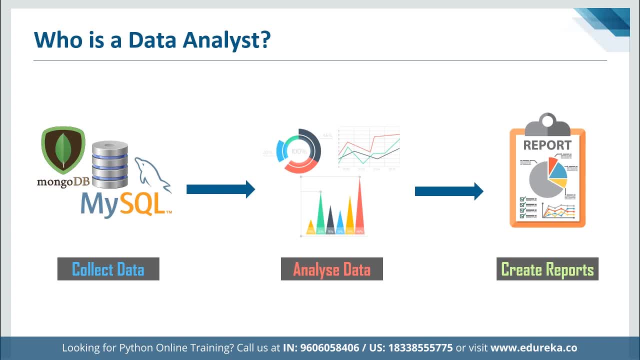 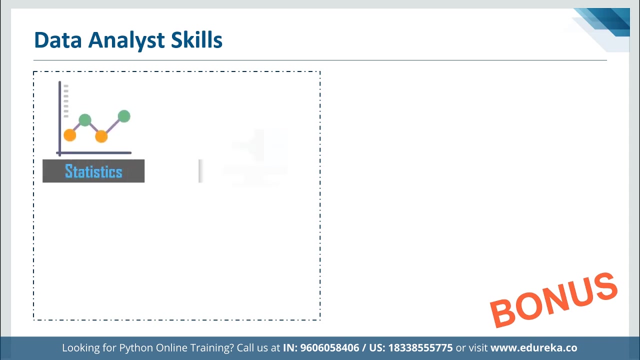 so they get the data, they analyze the data and use various tools to visualize, generate reports and give these reports to the management. sometimes these data lists help data scientists in organizing the data and giving the data okay. so what are data analysts? what skills a data analyst should have? basic understanding of statistics, okay, and knowing, like, how to clean. 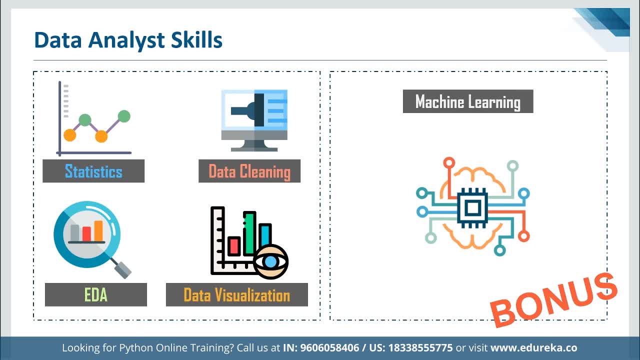 the data. basically, most of the data that you get in the real world is not super clean data. basically, sometimes you need to clean the data. most of the time you need to clean the data. okay, so those skills you need. then eda the exploratory data analysis that we are going. 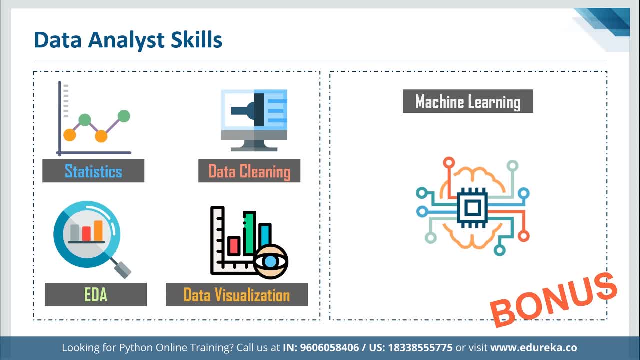 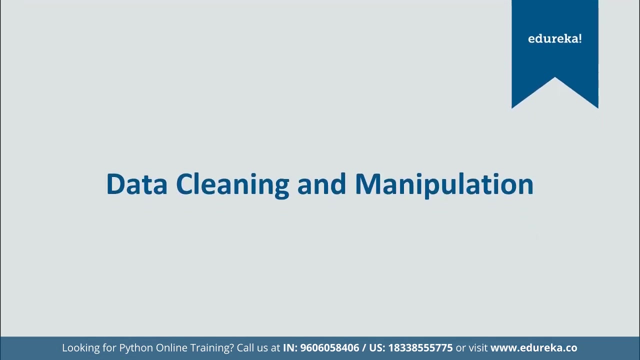 through today and the data visualization. this also will talk about a little bit about how to do the data visualization. okay, so machine learning is one aspect uh that uh data analyst will use, will have that skill and we will see today what are all the things that a machine learning unit does. okay, now we talked about data cleaning and manipulation. this 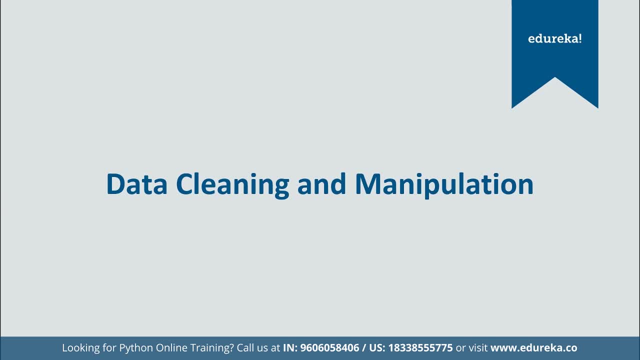 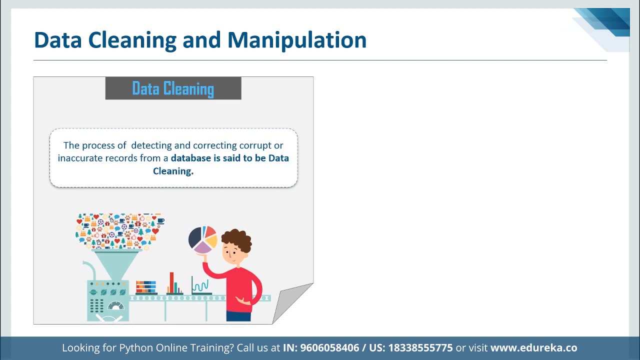 is a very, very important step. data cleaning is extremely important step because unless the data is of good quality, we cannot get the insights into that. even if we get the insights, it would be correct insights. so data cleaning and is the most important step. so what we mean by data cleaning. 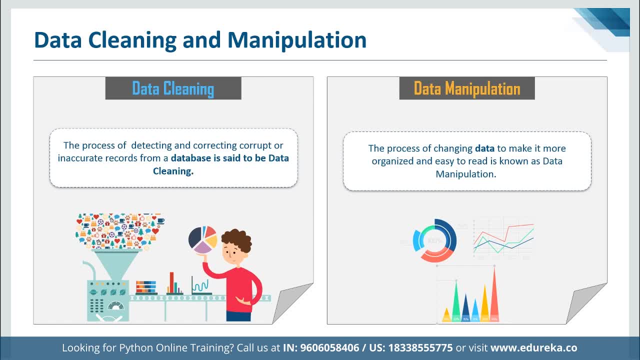 sometimes there will be missing data. that means, suppose you are asking a customer to enter all his information, his or her information. sometimes they miss some of the information which is not mandatory. okay, so that kind of information age is one like that, one way to gestimate the age of. 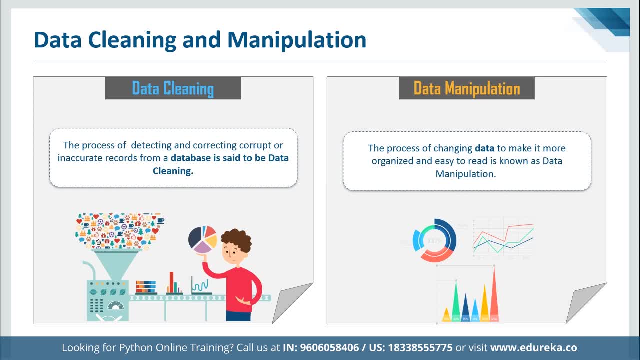 the product byう derrá advohu aprove. worry about if there is a surprising data will get better if you look at the data information- the his or her age, okay, so that is what the data cleaning is. today. we'll in our case study, we'll see how to clean the data and we'll take a real case, interesting case we'll take. 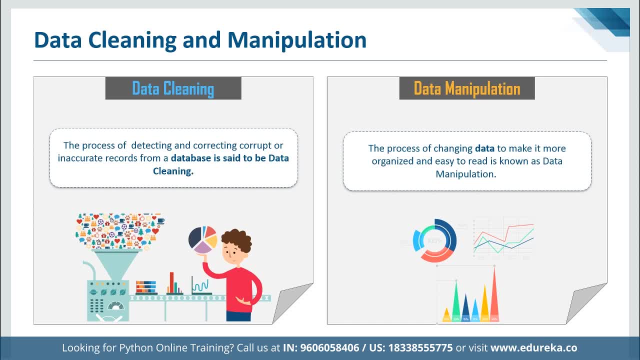 and we'll do that okay. so what is data cleaning? basically, it is a process of detecting and correcting correct or inaccurate records in the data. basically, you know that. what is cleaning? basically data cleaning to make sure that that is correct and has not having missing values. so that is what data cleaning is and what is data manipulation? the process of changing. 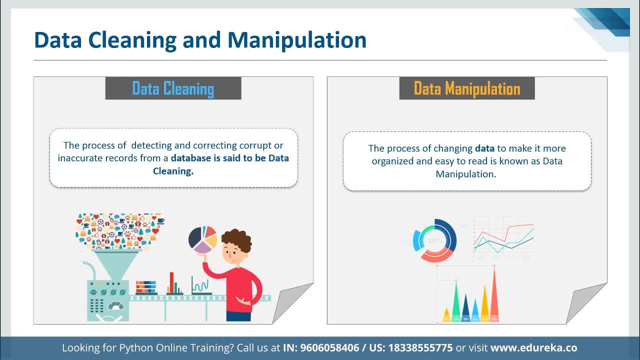 data: okay, as required. so sometimes there will be date and time. you don't want to see the time, so you need to manipulate it. okay, i don't want time now. okay, some applications, so you can just want to do some manipulation. sometimes you need to add some records together. you take a kind of sum of records and sometimes 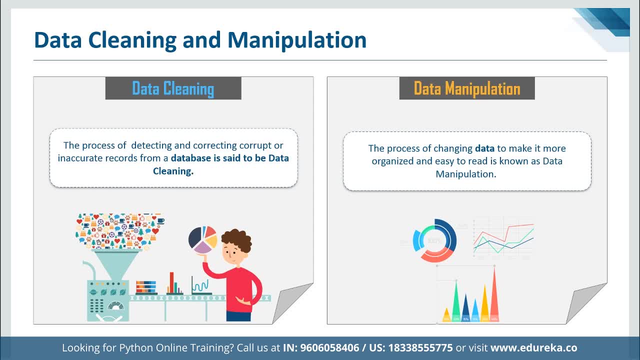 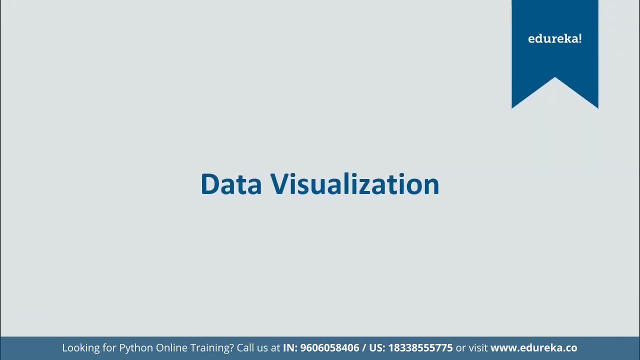 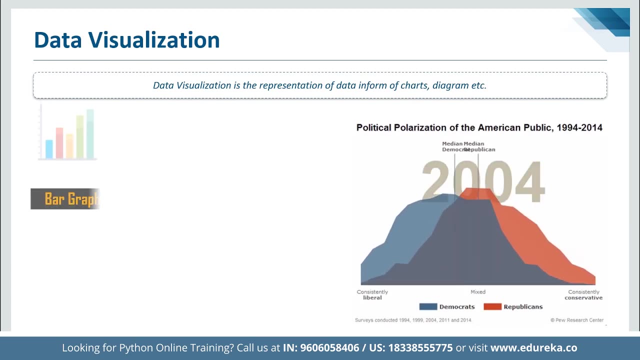 you need to just show the average of all these. things are data manipulation. okay, let us go to the next one and data visualization. so what is data visualization? it is an important aspect of eda, so we need to look at data at several perspectives. okay, there are 60 or 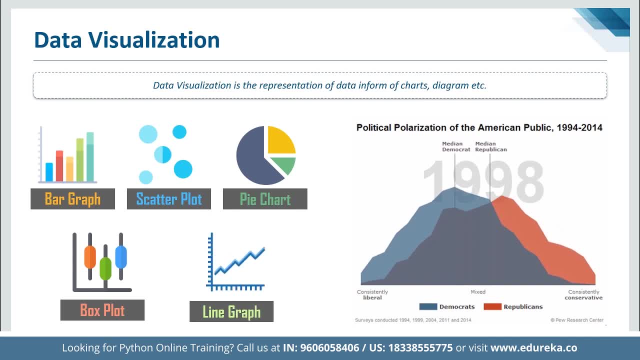 so 60 or 70 kinds of graphs are there, what is appropriate for your data? you need to look into that and use those things okay, so that you get with experience. basically, you need to use these things and see that what is appropriate for you. so, exploratory data analysis, we came. 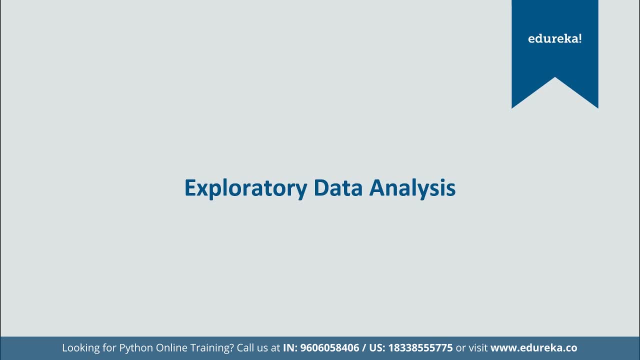 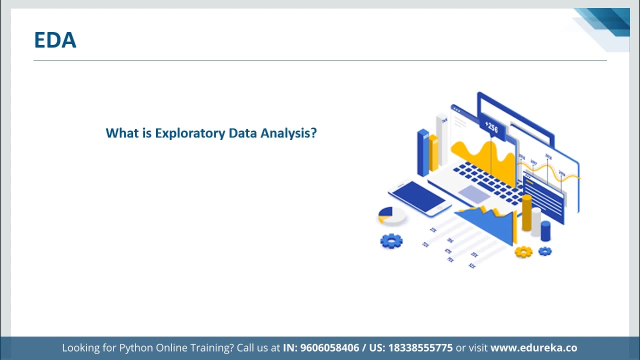 to the gist of today's topic. what is exploratory data analysis? basically, this eda, or exploratory data analysis, is a technique to understand all the aspects of the data, look at data from all perspectives and research into the data, whether data is correctly. just now, somebody asked: how do we? 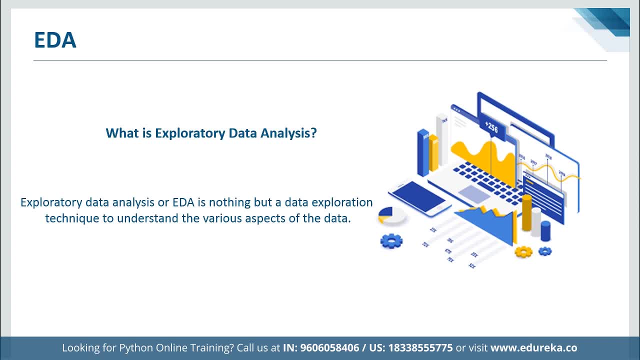 know if the data is correct. yeah, we have to do eda and we need to see that, uh, whether there are any outliers, what kind of standard deviation is there in the data and whether the data is normally distributed. a lot of statistical techniques are there that we 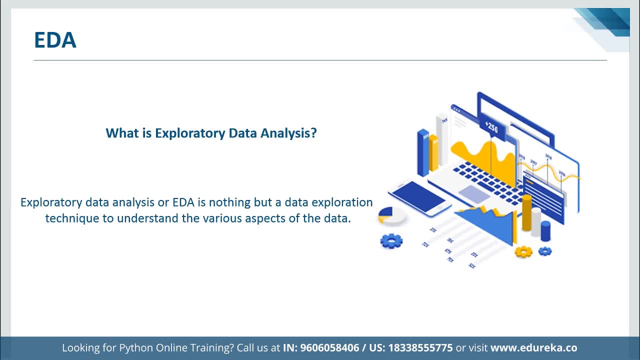 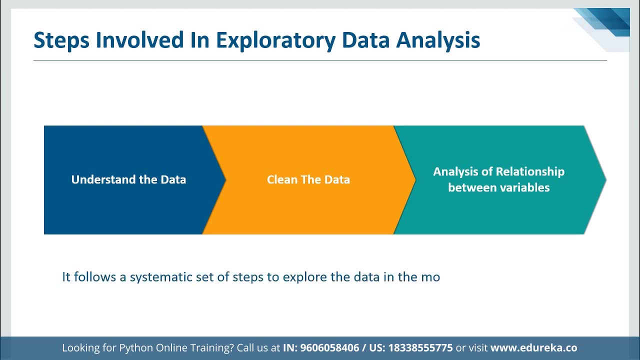 can use to see that if the data looks good or not. okay. so what are the steps in the eda? first, we need to understand the data. what all the features of the data? what kind of values the data can take? what is this data about? okay, all the details about the data. 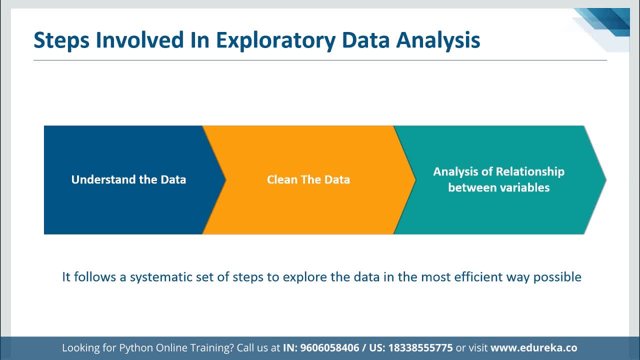 you need to know. then, once you understand that, then clean the data. clean the data means: are there any abrupt or outlier values for this data and are there any missing values? if there are missing values, how can we intelligently fill the missing values with reasonably close approximations? okay, then, analysis of the relationship between the variables. okay, that's what we'll. 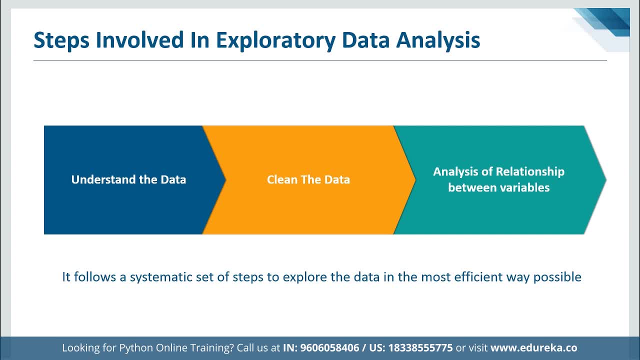 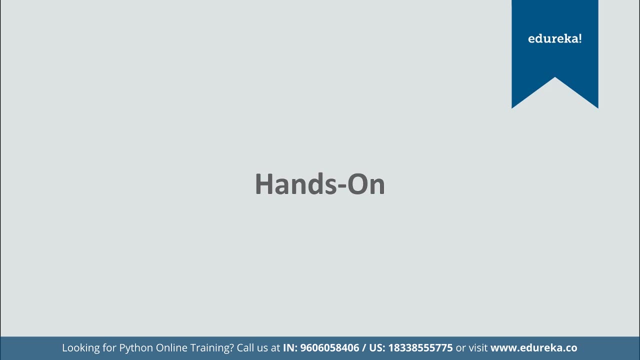 see today. basically, eda is a systematic process of looking into data and making sure it is of good quality. this eda step will take majority of the time for the project. suppose if we are doing project for two years- for more than a year we'll look into the data and analyze the data, clean the 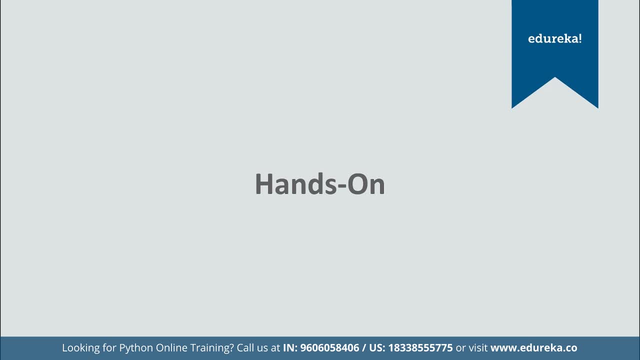 data. find all the missing values, find all the data about the data. that is the major aspect of the eda. okay, so let us go to hands-on and let us look at one case study. okay, let me go to this python here. let me go to this python, as i said. okay, so these 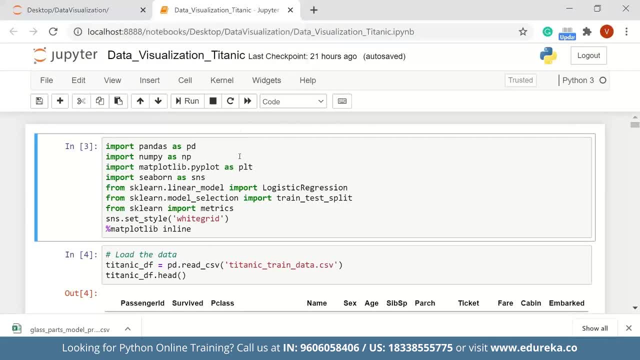 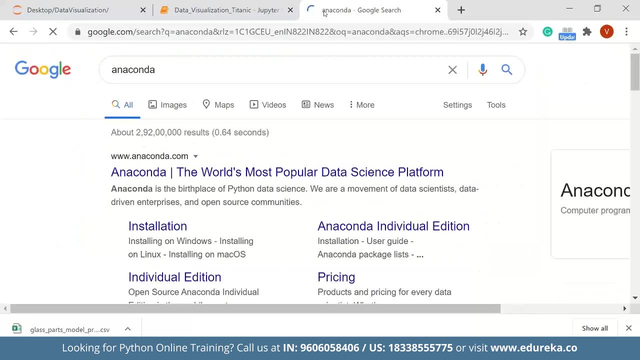 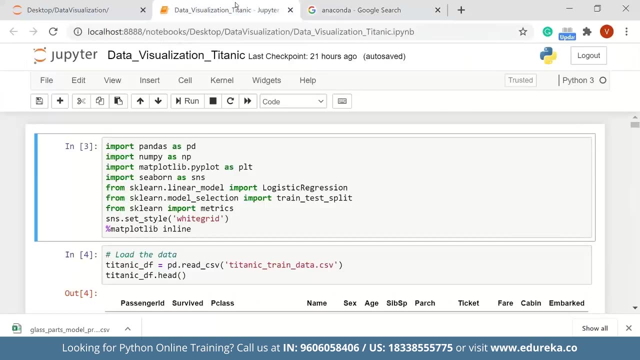 are open source for python. we are using python here, okay, so there is something called anaconda. if you download that, you get all these tools. okay, so this one is the most popular platform. if you download that, you will get bunch of tools. one of the tool is this: jupiter notebook. 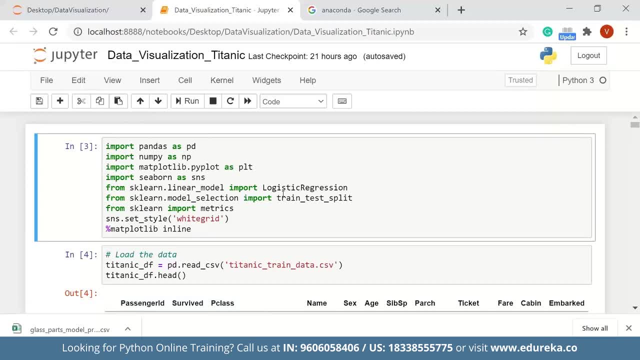 so what is this? jupiter means ju stands for julia. jupiter sounds like or julia means jupiter or julia means jupiter, because jupiter means julia and jupiter means jupiter and jupiter. that is a programming language that you can use this tool for ty. t stands for python. okay, you can. 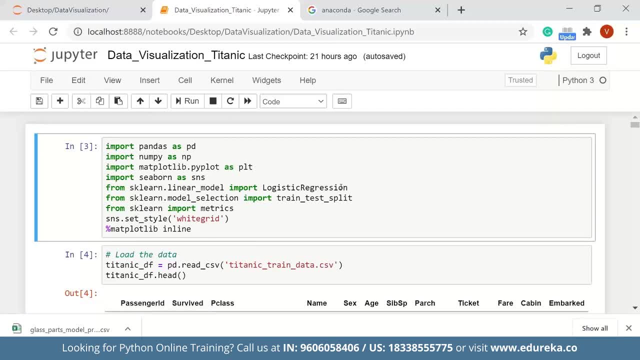 use this one for python also, and r is for r programming, like there is another popular programming language called r that also you can use. so for these three languages you can use this interface. this is extremely easy to use interface. so basically, if you download anaconda, you can open. 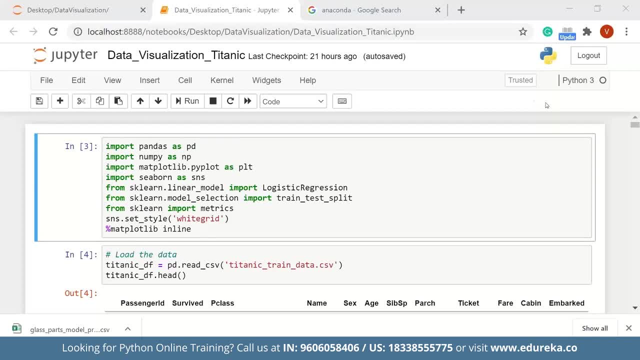 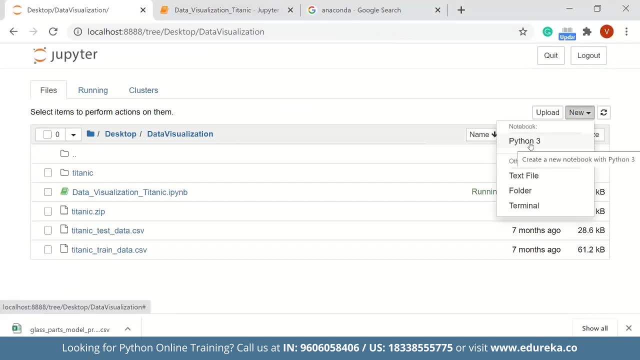 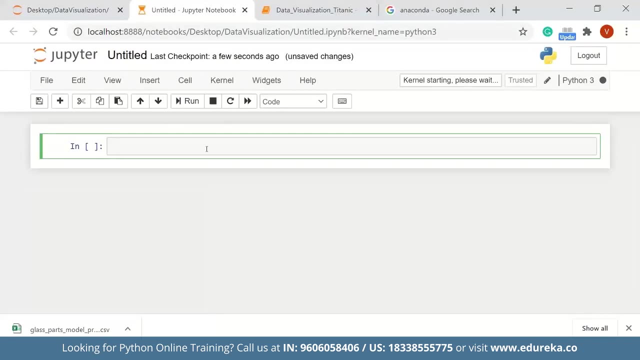 this jupiter. so basically it is just a cell by cell kind of thing. suppose, if i want to use a new notebook, if i say new and python 3, python 3 is the latest version, 3.78. okay, if i say that it will open a new notebook. so here if i do anything, each cell by cell, it will execute. if 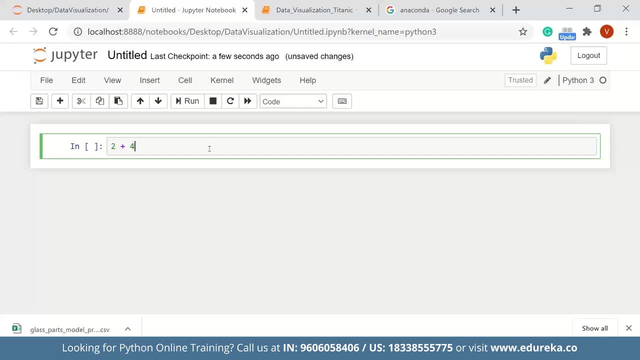 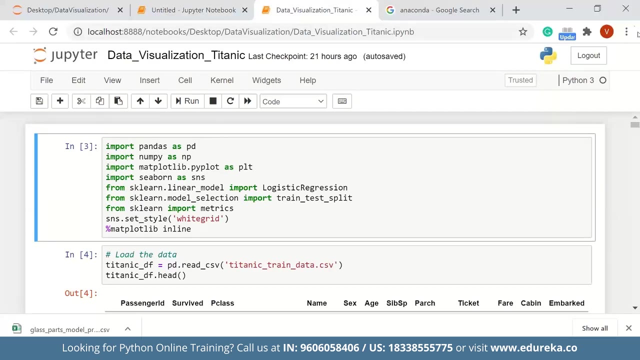 i say 2 plus 4, okay, so basically it will execute cell by cell. okay, if i write anything code, it will execute that for all these three programming languages. then you can name this and you can all do this extremely easy programming interface. basically, if you want right programming, python. 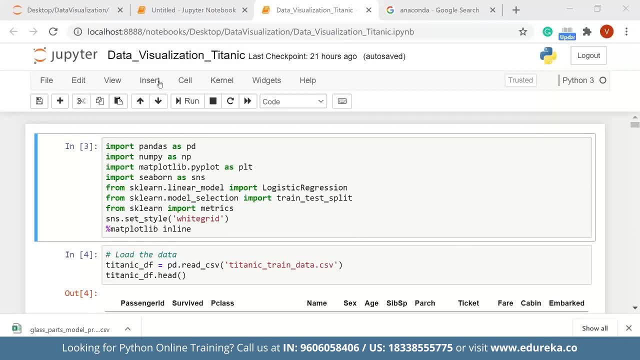 the easiest way is to start this one to get this one. okay, so there are other tools here. a spider is there. there are other tools. this is the most beginner friendly interpreter. basically, okay, is good knowledge of statistics required to learn eda? the basic knowledge of statistics we all have. you all know what is average, what is mean, what is mode. 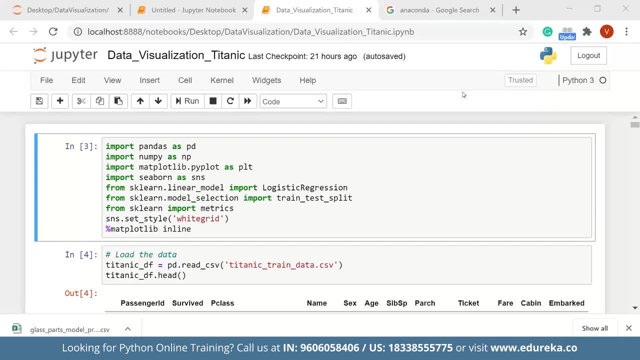 all these things. if you can have good statistical methods, that is always useful, but it is not much required as long as you know what is standard deviation, what is variance. all this is high school math. basically, if you complete high school, you have enough statistical knowledge. okay, so you? 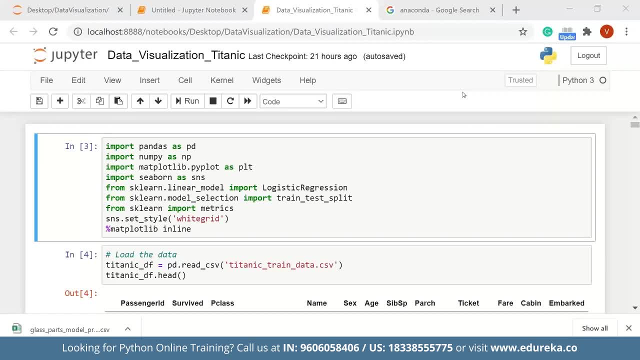 don't need any specialized degree in statistics, or that's it? okay. so that's the basic knowledge of statistics we all have. you will all know what is average, what is mean, what is mode, all these things. okay, so this is basically the environment that we use here. each of this is called cell. 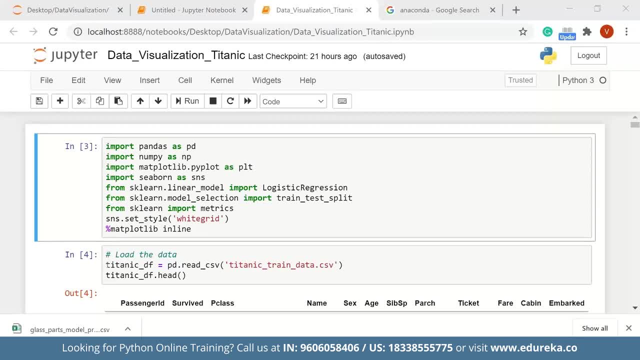 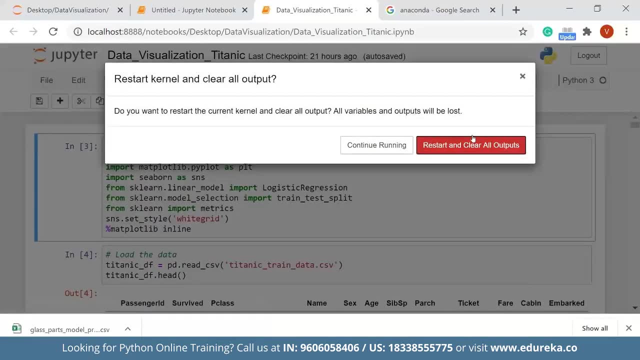 okay, so basically this is one cell. you can see that this is second cell like that one. okay, so here we can say that kernel is the engine that runs it. if you want to restart, you restart. okay, so this blue means it is basically. you can see the blue. 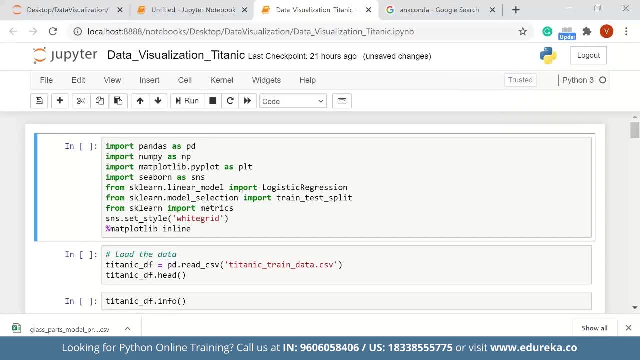 here. so that means it is in the command mode. when it is command mode, you can create cell mode, create cells. if you say yes, if you press a in this command mode, it will create a cell. i'm pressing a now so it will create a cell above. if i keep on pressing it will create. 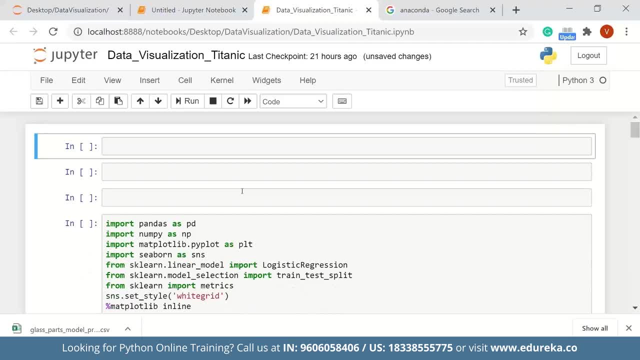 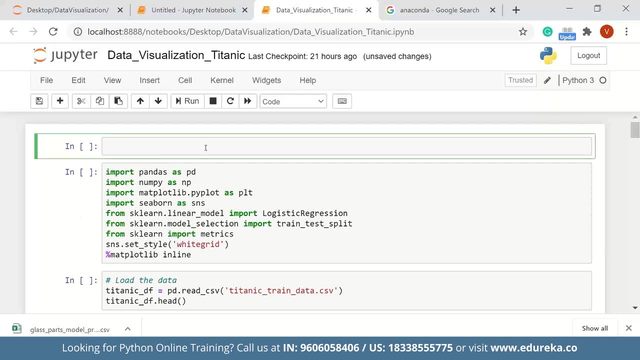 all the new cells. if i press dd, it will delete it. simple steps here. okay, so if i want to put some heading, i can put like: okay, let me put a heading too. so here it is saying code. i want to say markdown so that i can use it for a heading. so heading starts with this. 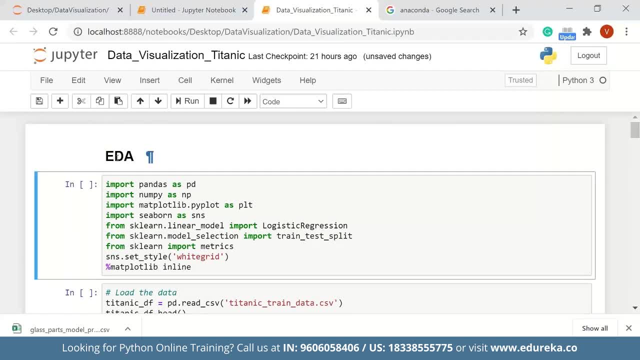 so let us say dvd. so this is not executable code, this is kind of headings and all those, all your kind of help, all those things you can provide here as a markdown. okay, you can put equations, you can do anything here, okay. so if you want to put a equation, basically, 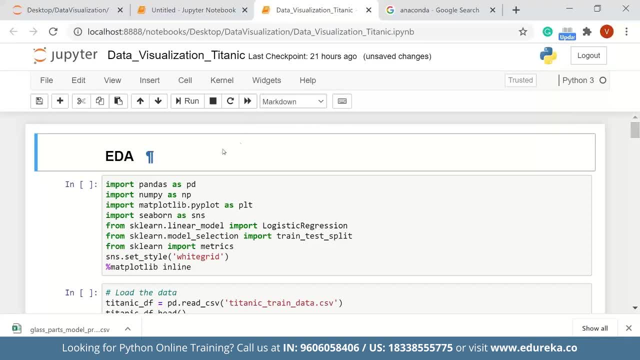 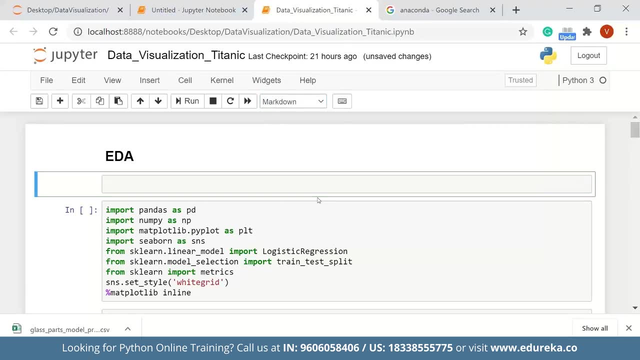 what you need to say is basically: you can use that one, so if i press b, i can open another cell. if you want to put an equation, all you need to do is do this one and basically start with a dollar and say that a equals b squared something. 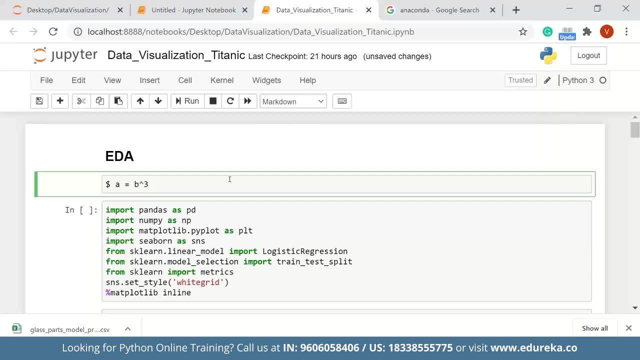 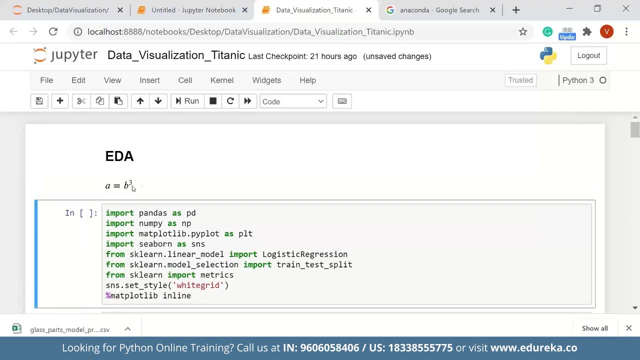 like that, or b cube, something like that. okay, you can put integration all kind of any kind of mathematical symbol. you can do that, so it will put all these equations root, square, square, root, all kinds of mathematical symbols. you can do that, so it will put all these equations. 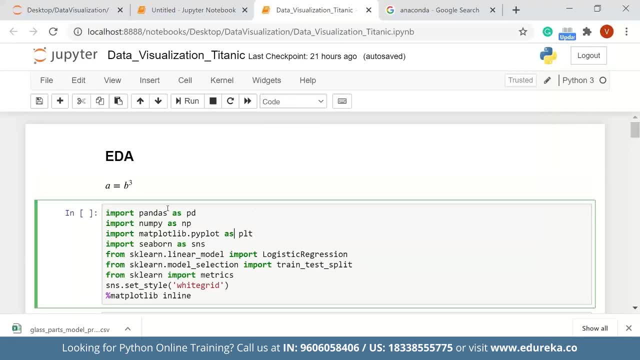 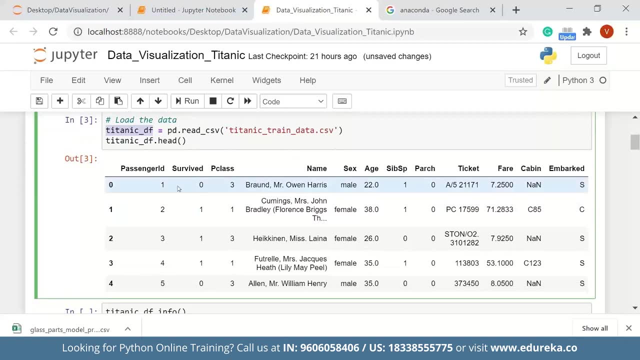 together and you can use it here like that. okay, so data frame is like excel sheet, almost okay. so how it will be? it will be like this one. so passenger id is there. survived zero means no, that person died in the accident. survived one means that person survived the. 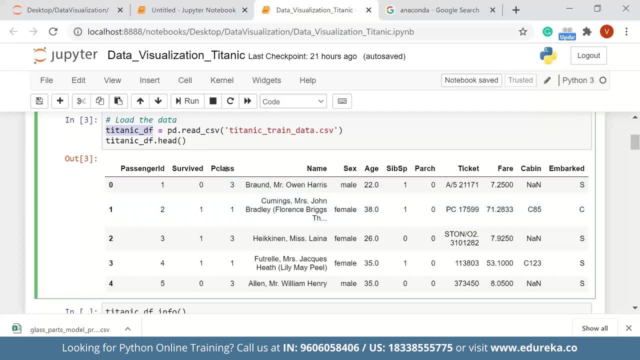 accident means they lived after the extent. what is the passenger class? what class they boarded on the ship? there are three classes: first class. second class, third class. okay, Okay, what is the name of the passenger? What is the gender of the passengers? Is it male or female? What is the age? Where they embarked, Where they get on the ship? Is it Southampton, Is it Cork? All these data, So this is the data basically. 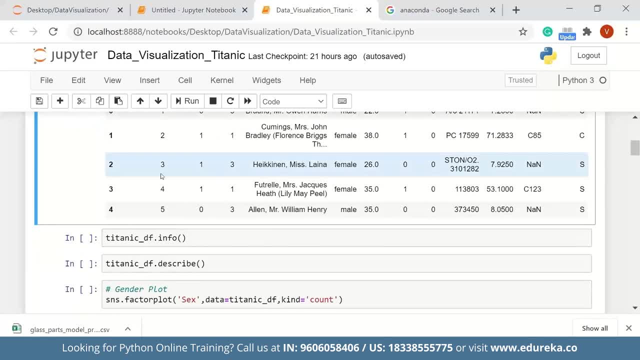 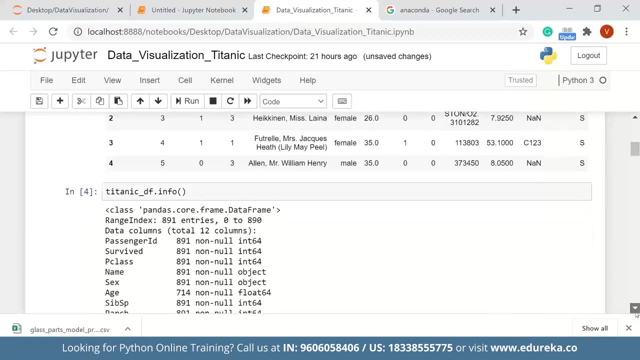 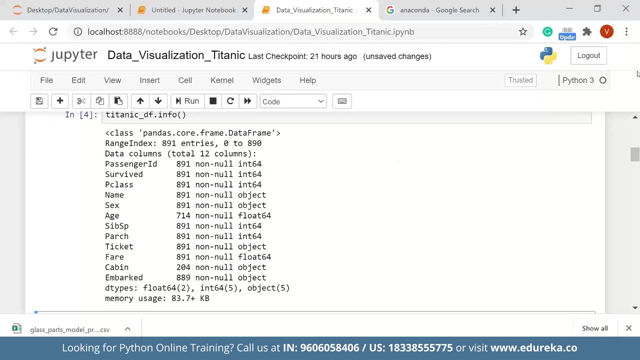 Okay, once you get the data, now you can see that. what is that data? Can we get the information about the data? Okay, what data types it has, all those things. So, once we get all the data about the passengers. So basically, what is our problem statement here? We know that this many passengers went on the ship and some survived and some did not. 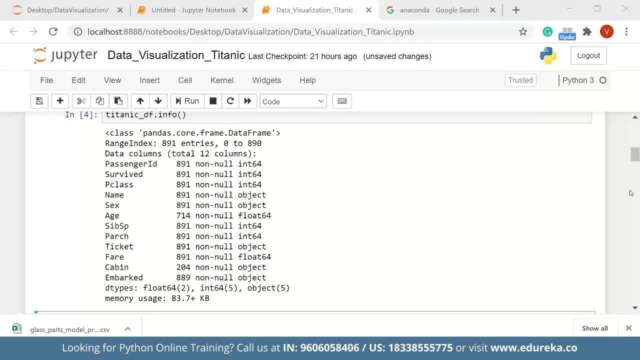 So if I have a new passenger now, okay, that went on that ship, Okay, and we don't know whether that person survived or not. We have to predict whether that person survived or not. Basically, we need to know what is the probability that person survives if that person gets on that ship. 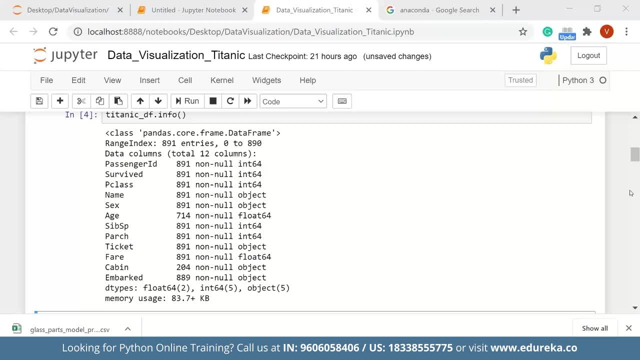 Suppose XYZ person: okay, bought the ticket and did not make it the journey, So got a little bit delayed, did not make it, So would that person would have survived or not? That is what we are predicting here. So that is the mission line. 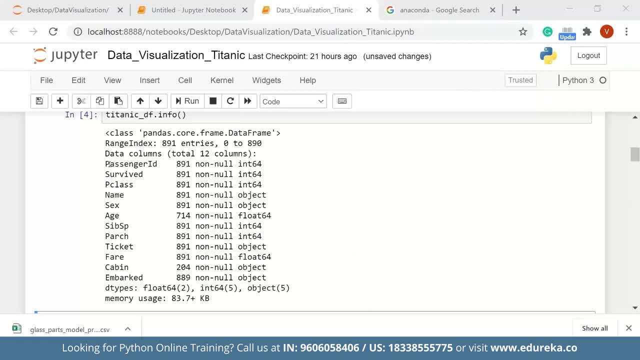 learning problem that we are predicting. Okay, So we got all the data. Okay, So what is this? data tells us we have integer column for passenger- it is survived or not. And object means we know string, because name is not甜, This is string. 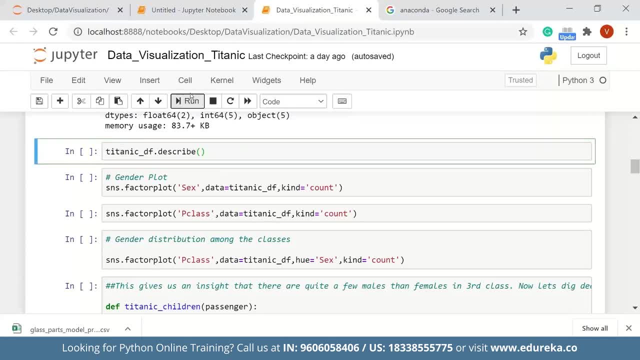 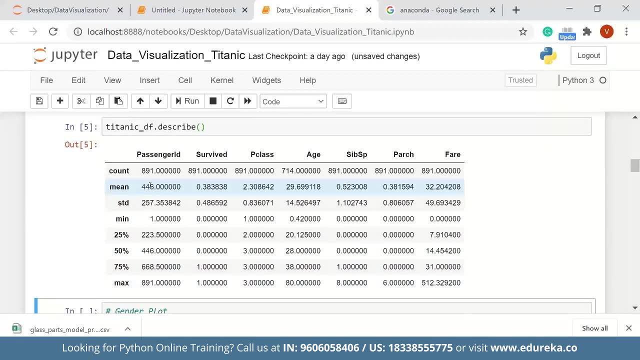 Okay. So now let us say that. what is this data Looks like? okay. so These are the statistics about the data. Okay, date items are there. that means 891 records are there? what is the mean passenger rate? what is the standard deviation? what is the minimum? what is? 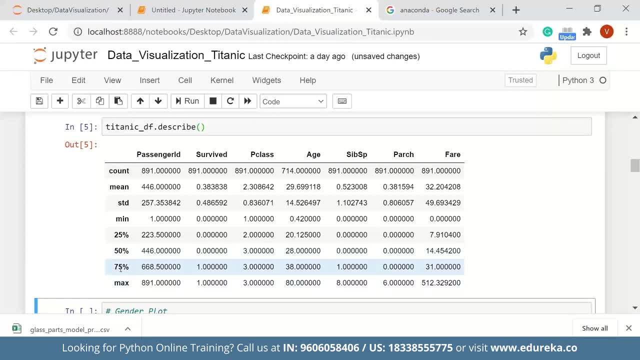 the first quartile. what is the median? what is the 75th quartile, third quartile, what is the maximum data in that one? so if you take there 891 British pounds, I think this one currency is the highest, the number of record. what is the mean it? 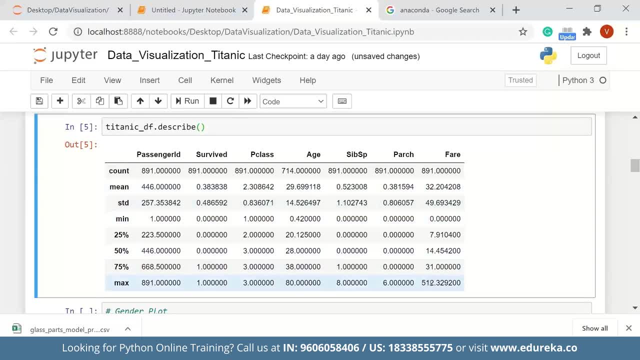 is 32 pounds. what is the standard? 49. what is the max? somebody paid 512 pounds and what is the minimum? so somebody did not pay this zero, okay. what is the 25th quartile and all? what is the median? it is 14. all kinds of data you get. what is? 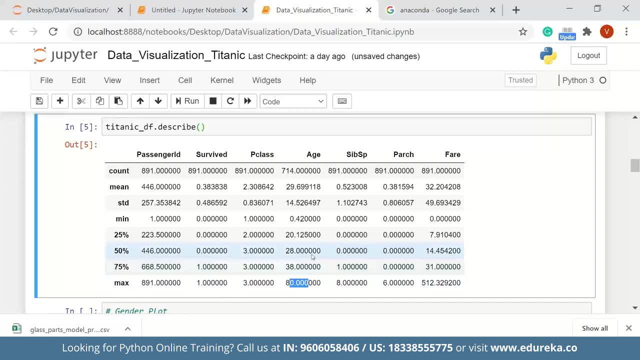 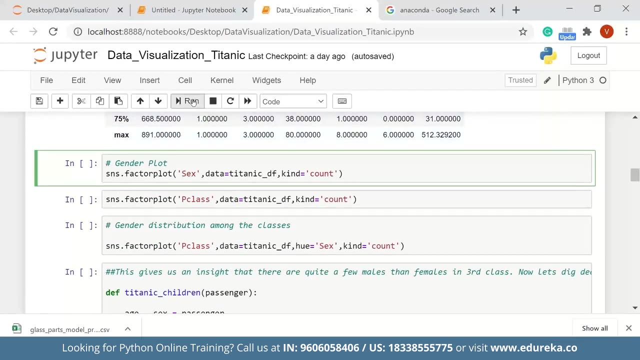 the highest age of the passenger: 80 years. what is the lowest minimum age? a few months old, less than a year? okay, all kinds of data you get here. okay, let us go to the next one. now we need to analyze the data. so basically, we need to. this is the seabourn package. we 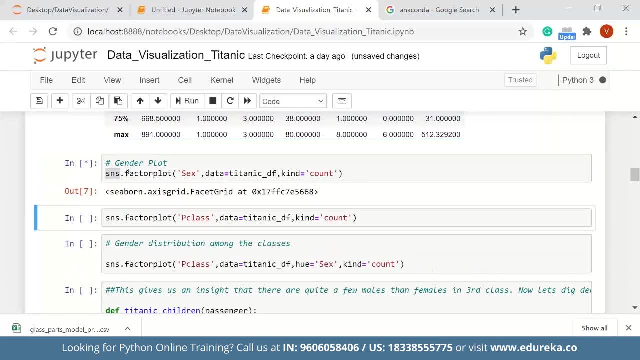 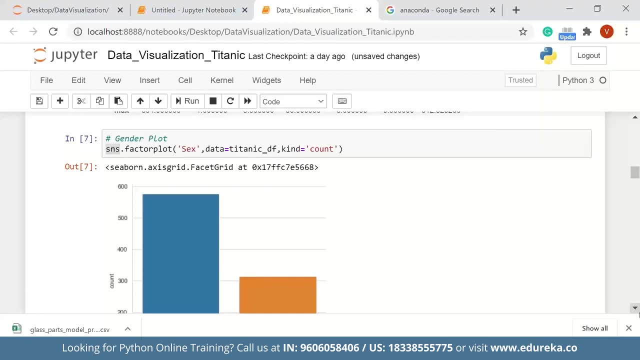 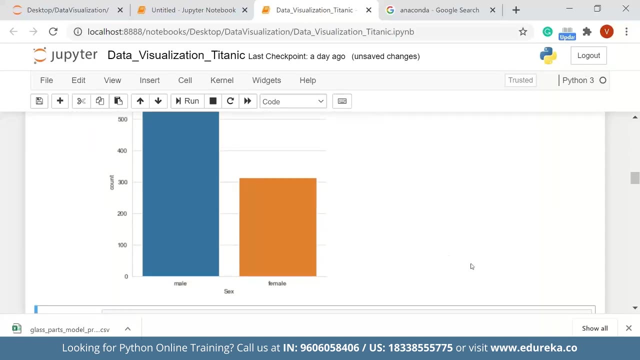 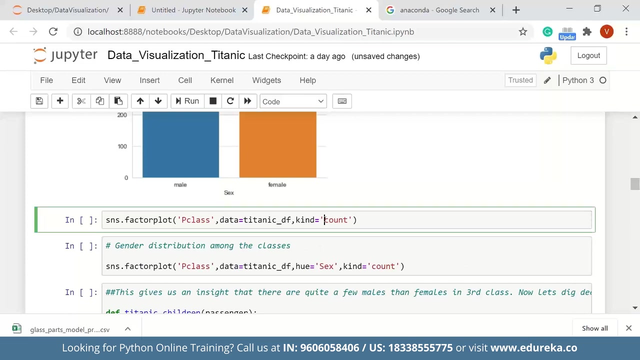 are talking. this SMS is the seabourn. okay, we imported seabourn package so that will plot us on various aspects of the data. so you want to see the gender, sex, how many males and how many females are there. so males outnumber females here, okay, and we want to see that. what is the class? 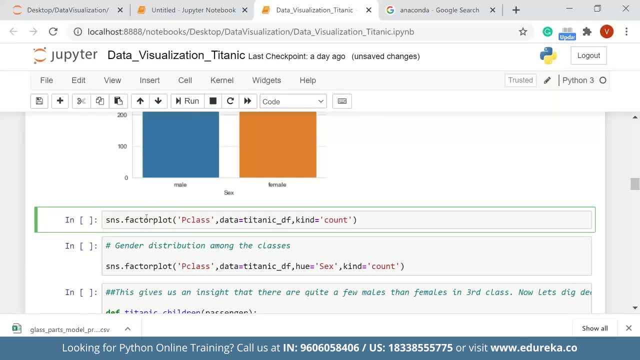 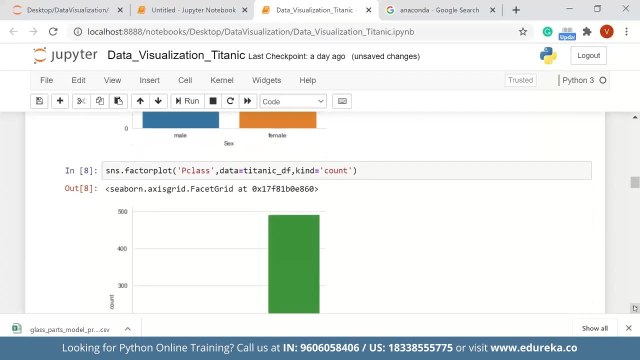 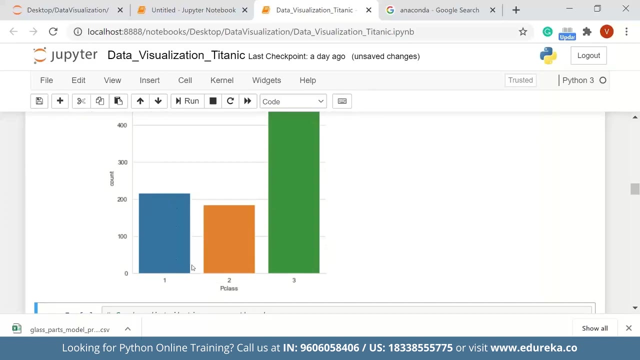 wise. first class, second class, third class, how to do that? just if you mention the plot name, the package can do the plotting. that is the beauty of these packages. so now there are like about more than 200 passengers in the first class, then second class, not that many, but third class has most of the passengers. 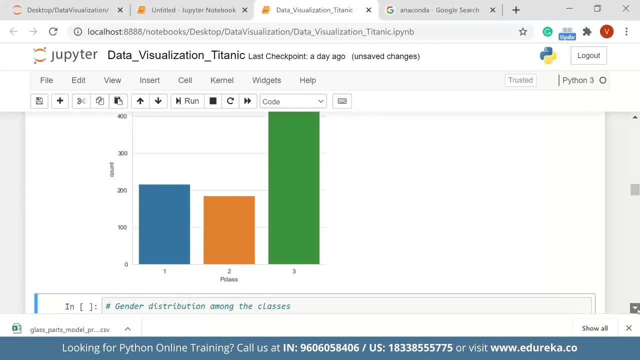 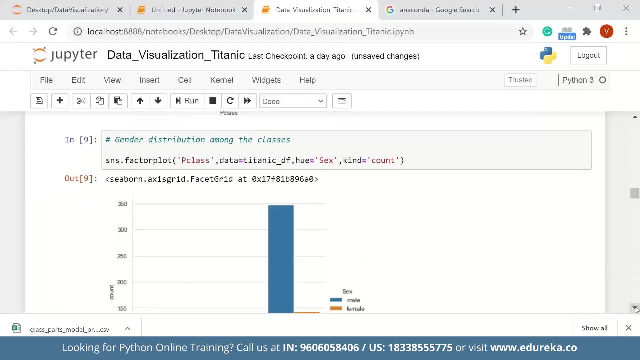 okay, so then again, you can see that. okay, what is the distribution of the passengers by class? okay, so in the first class there are more males than females, even in second class, when in third class there are very few. the ratio of males to females in the first and second class is close, but it is very different in the 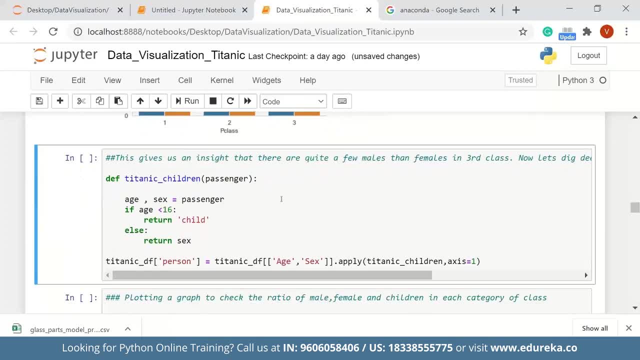 third class. okay, then the data manipulation. these are the things that we are talking about. then you can write a simple Python functions and all this is the way to write out function will say that: okay, let us see how many children are there. okay, let us assume that a child means less than sixteen years, so we can write a method. 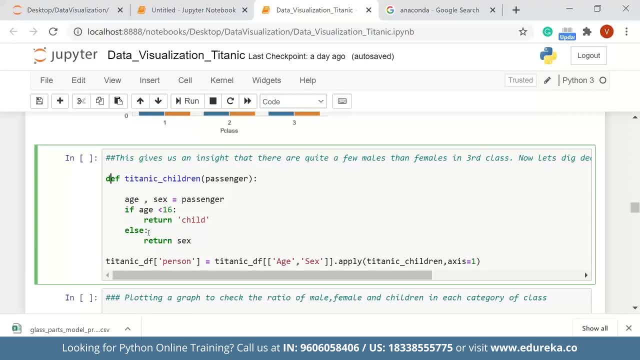 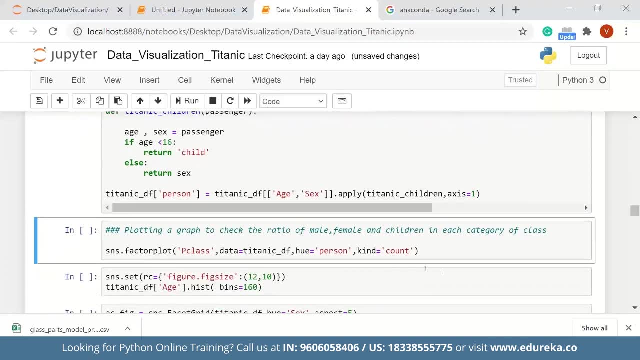 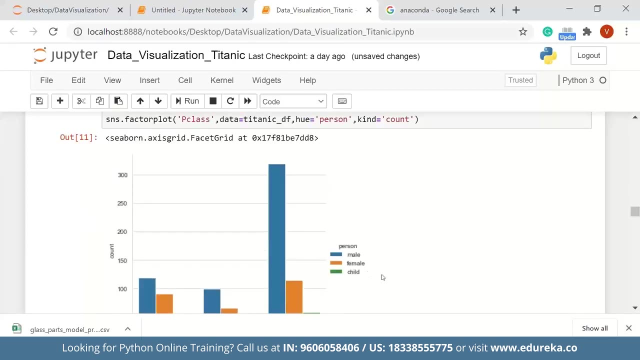 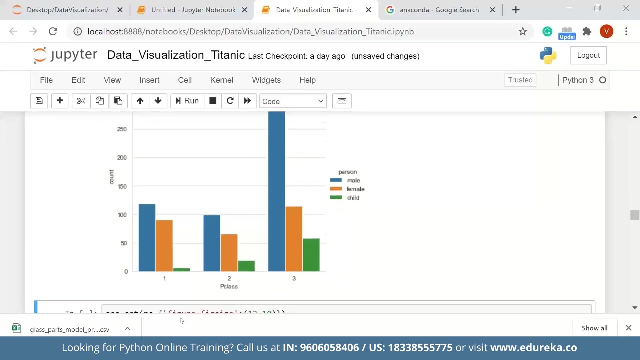 like this one and say that this is not just males and females, we can have children also. so let us see that. how many children are there? okay, now let us see that t class count. okay, now see, we got another dimension of this data: that males, females and then children. okay, you see that very few children in the first class. 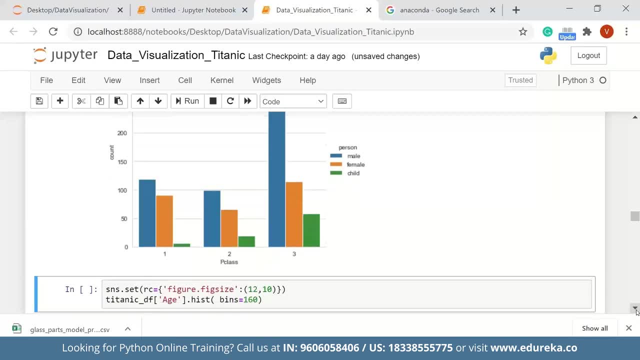 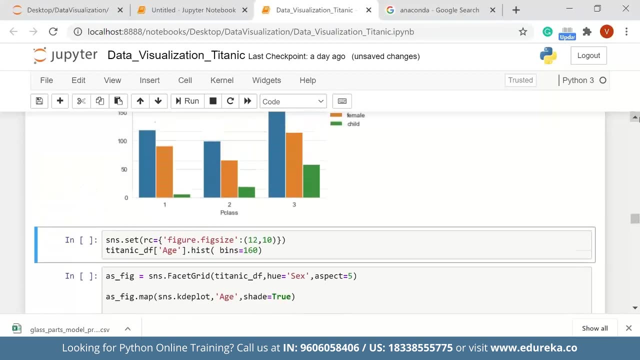 but many more in the second and third classes. okay, so this is all the steps that we are talking about in the data eda. okay, all kinds of aspects of data should be looked. we created another kind of data here- children- and we saw that. okay, who is less than 16? we call them children. this is 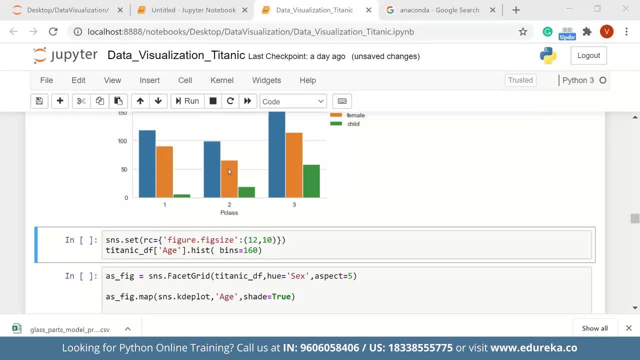 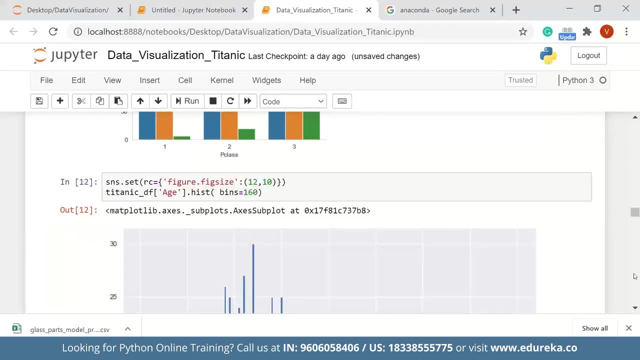 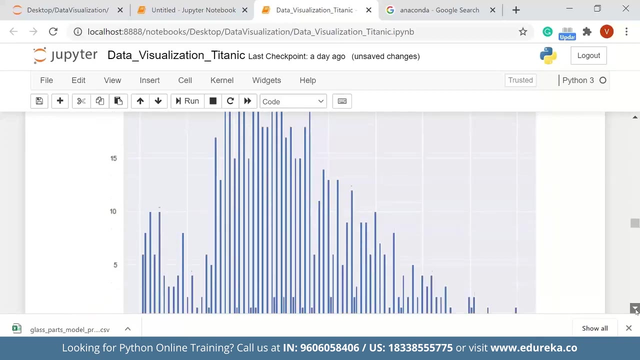 all the data analysis, we are saying, okay, so first of all, age is not there for all the people. this is age. we need to do that. so how to fill the age? because some people age would do not have. so how to estimate age for all the passengers? so here we are plotting age for all the 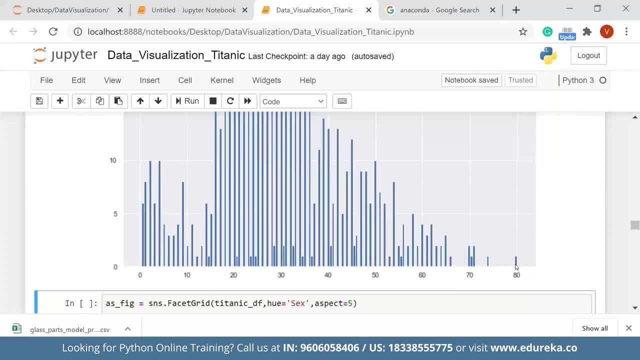 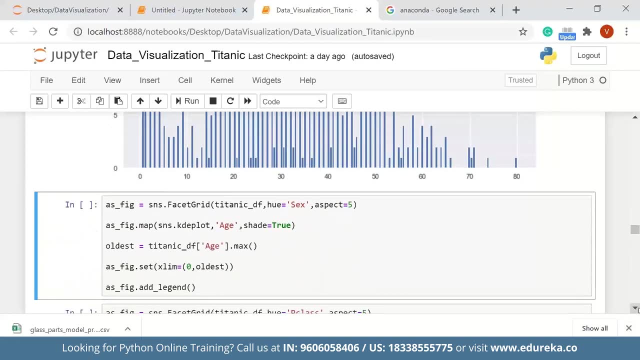 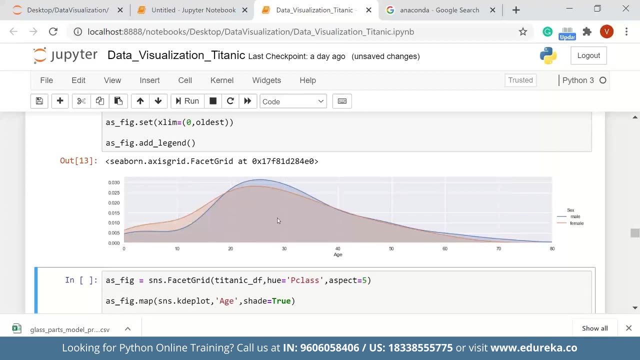 people. we know that 80 years is the oldest passenger- okay, and youngest passenger is only few months old- okay. so we know all that data. now we can look at this data manipulation and distribution. so this, these are all the statistical ways that you need to look into. so if you put for a small kids 29 years age, 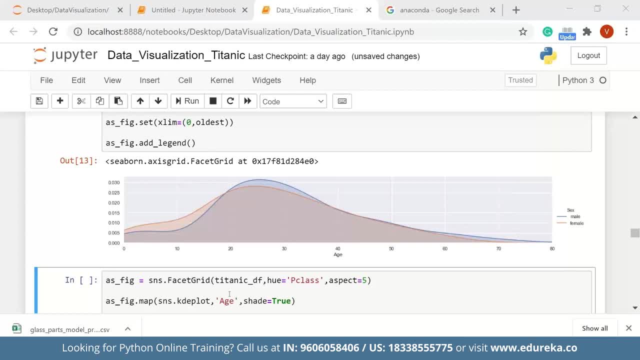 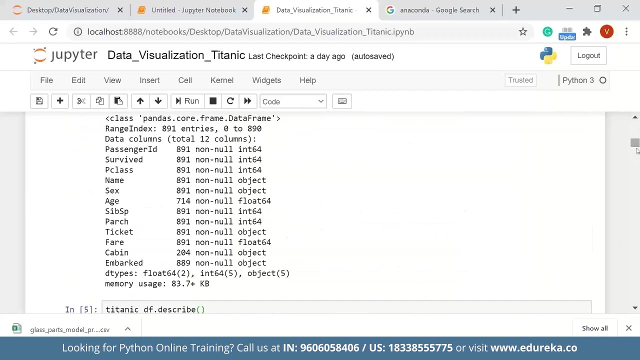 then that won't be correct, right. so that is why we are doing this processing. this is all the exercise that will go for complicated data set. it will have millions of the data and hundreds of features. by the way, these are all called features in machine learning terminology. these are all called features. so 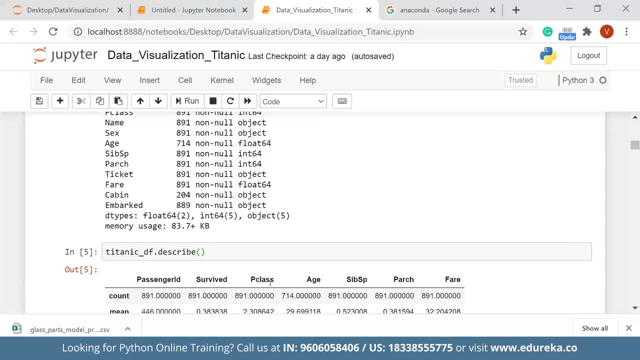 basically these are all features for us. passenger ID survived three, four, five, six, seven features. we have fair parent-child relationship, sibling spouse age. these are all features. here we have seven features. in reality we'll have thousand in the real data. okay, so doing the EDA is not that easy, okay, but it will. 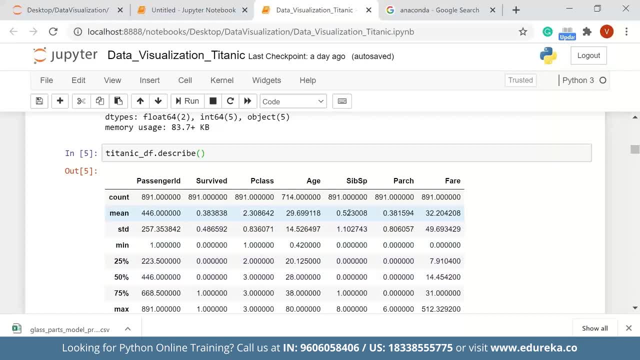 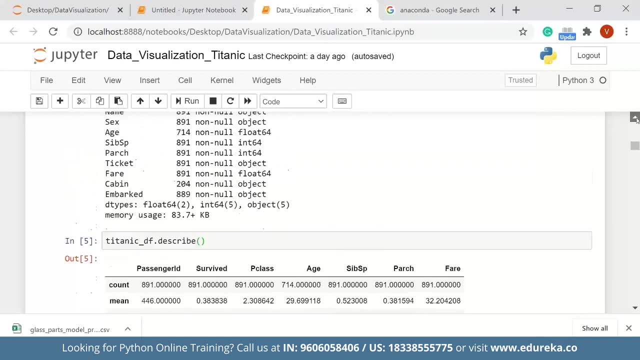 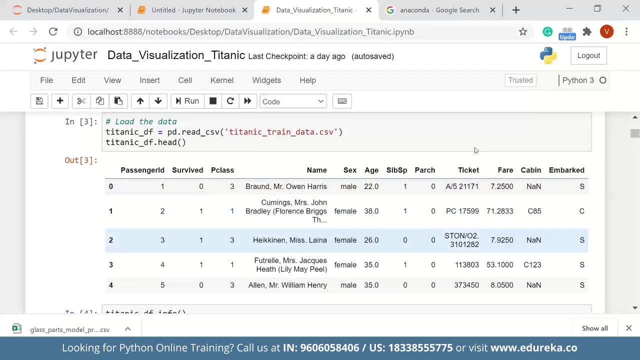 be easy in the sense that we use all these things- insights into data- but it will take time. okay, the describe did not give all the string value of that one. let me show you the data here. this is the correct, okay, and the describe. you don't see the name of the data. okay, so this is the correct data. okay, and the. 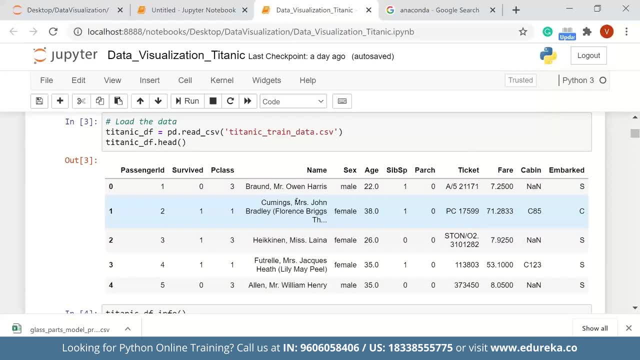 give you the name because of the OkeStream, because standard deviation and all is not possible. and strings, because standard deviation and all is not possible, and strings. that's why it didn't view. so can you see the name and all the column and can anybody tell me what is the best way to feel the age of? 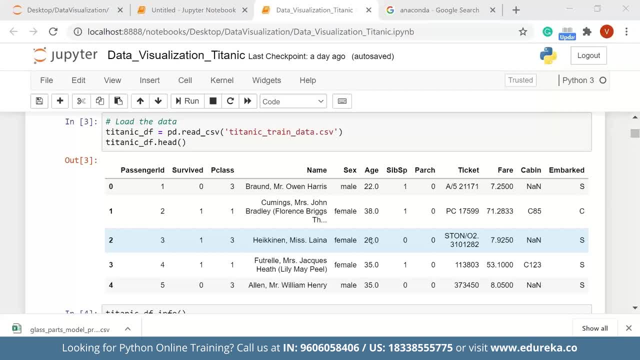 missing value. so some preprocessing is needed. this is what the pre processing is needed. this is what the process simply are talking about. you have to use the rest of the years end funds and another feature and estimate days. what you have to use another feature and estimate the age. what feature I can use? 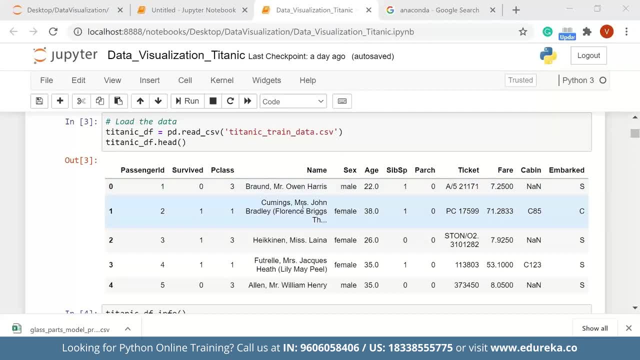 If you see here for name: Mr and Mrs are there for adults and Mrs and Mr are there for kids. Okay, so for young people there is another title, basically, if you see the titles basically, 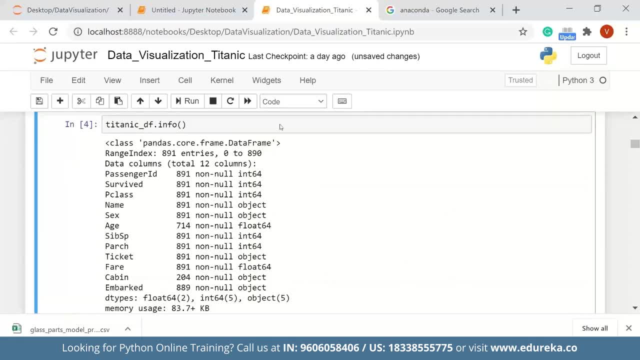 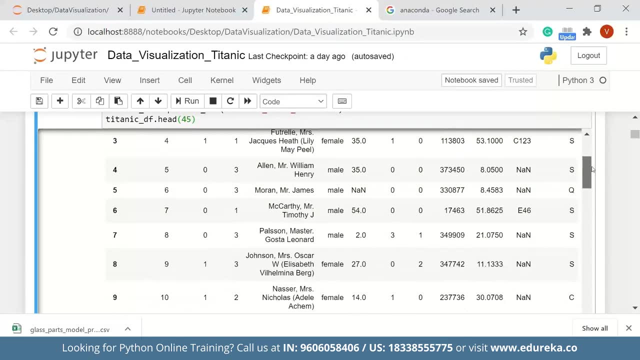 You can put here 45 or so to see a lot more details, and you can see that other titles are there. So from the title you may get to see here there is a master, That means he's a young person, okay. 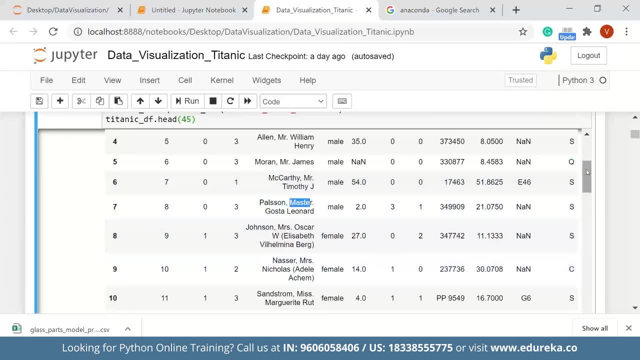 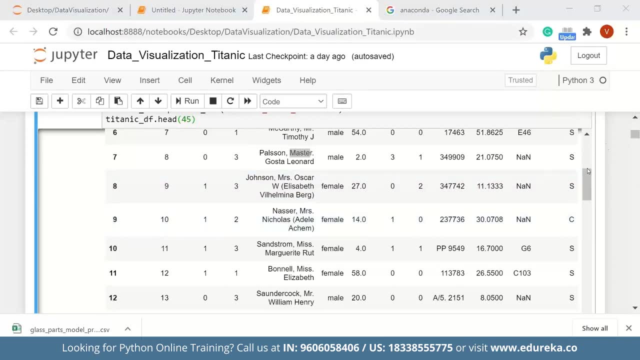 So we can divide the data into adults and children and then take average of the median of the children. okay, to get a very good estimate about the child's age. If the data is missing in that category, where there are master and young people, you can take their data and take the average. not the entire data and take the average. okay. 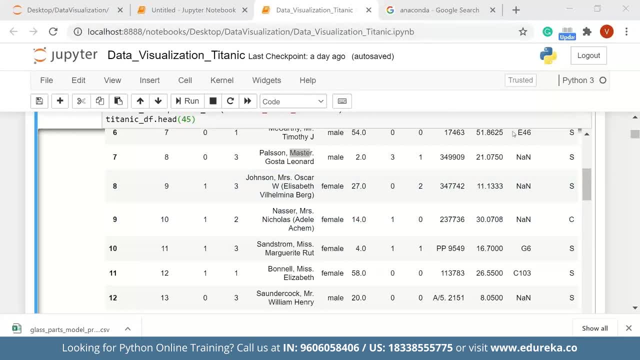 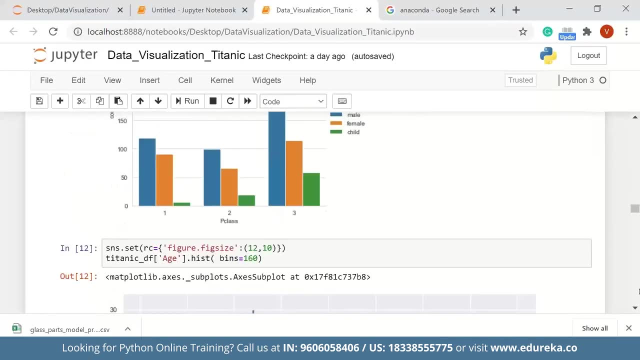 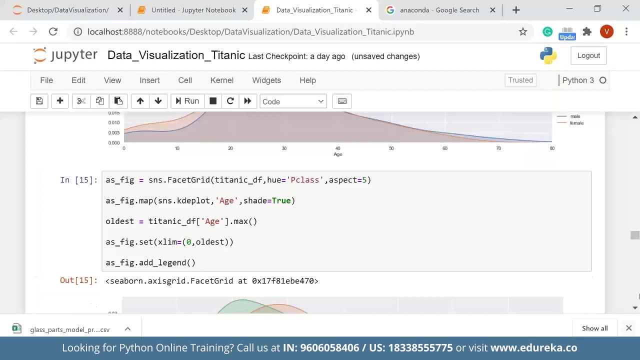 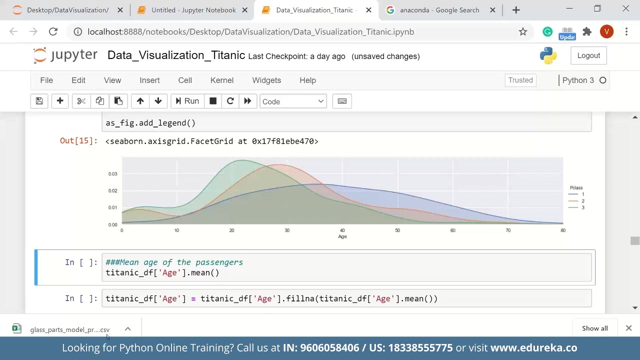 So, basically, those Are the insights that you need to have to have good data manipulation. So we'll go further. basically, we'll look into all these things. These are all the things that we need to look into. Okay, so again, the distributions we need to plot so that we will see what is the data distribution here. 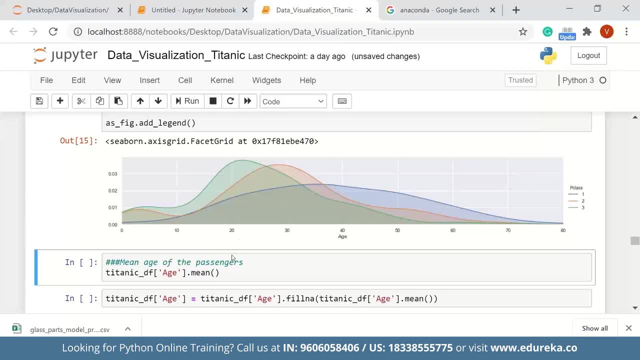 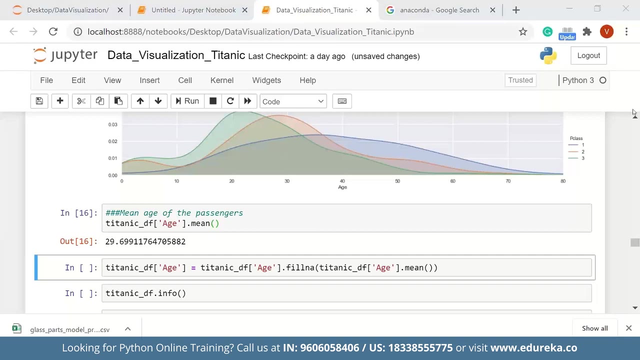 Okay, what is the distribution for each class by age? Okay, what is the mean age? Basically, as I said that 29.69 is the mean age for all the passengers where we got the data. Okay, so now comes the question: how to build the missing values. 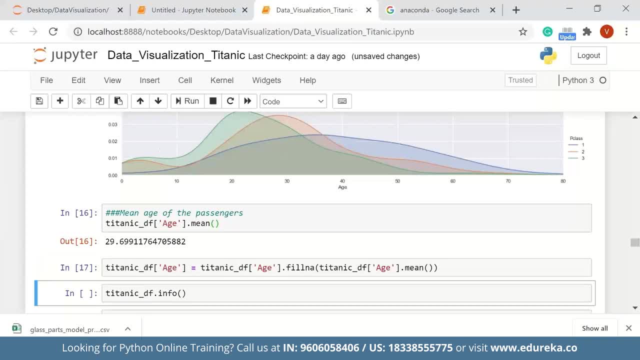 Okay, this is the crude way is basically, if you put this one, okay, if you say that wherever there is no age, take the average and put the age there. that is a crude way of doing that we discussed. that is not the correct way. we need to get the names. 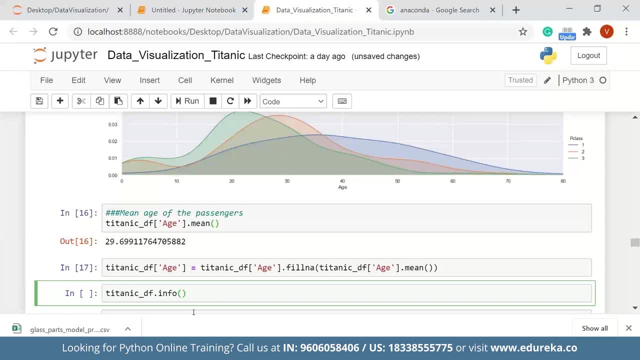 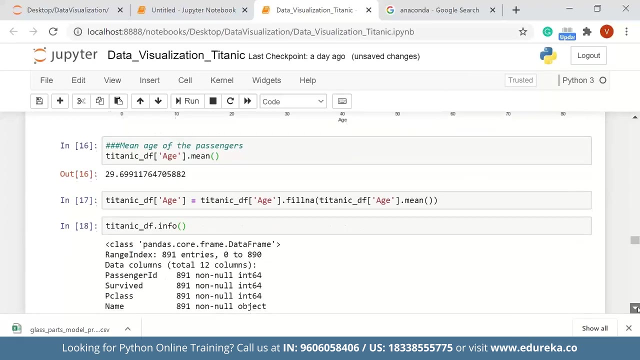 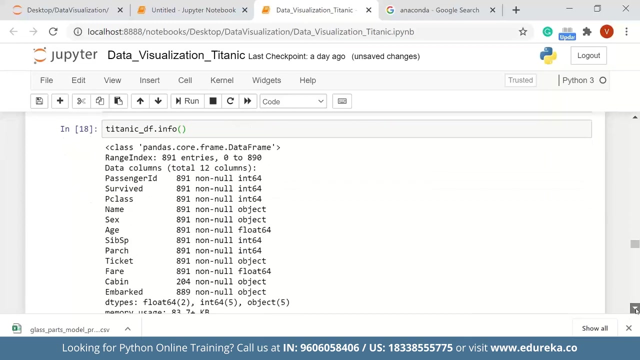 I'll give. Put the passengers into different categories and take average or mean or median of those categories. all the kids, average ages. you can take media. that is a good way. So this is another way, if that kind of problem is not there, so you can use this kind of code to put the values for that. 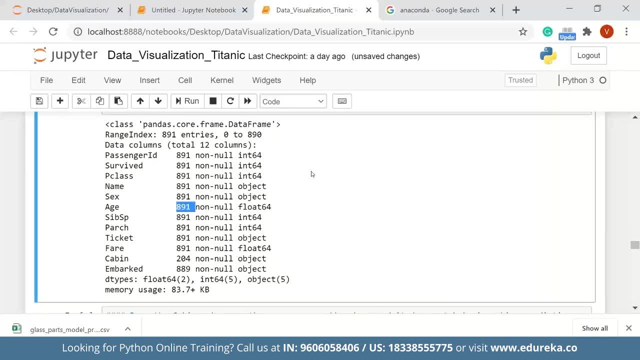 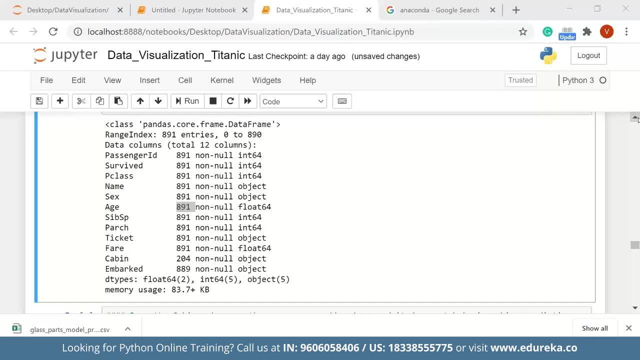 If you want to go further, then you can look at all the titles. some are doctors, some are. there are several titles. So if you split the people into their professions and the titles and all those things, then you will get even better average, better estimate. 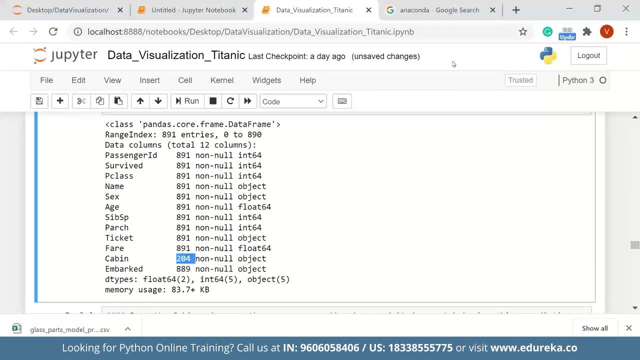 So if you split the people into their professions and the titles and all those things, then you will get even better average, better estimate. Now here cabin has missing values. Now we need to talk to the business and say that does cabin add any value in figuring out this one? 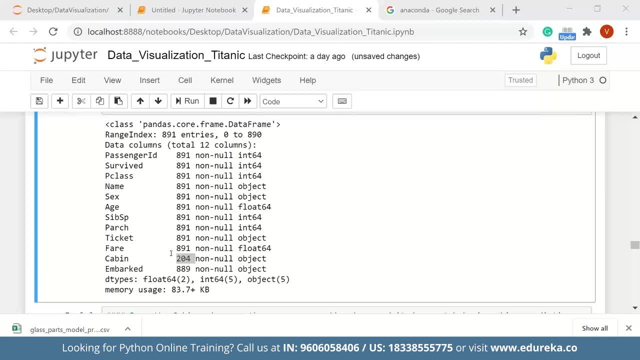 And the other problem we have with the cabin is only about 25%, or less than a quarter, has this information. Does it help us or not? Okay, if you really think that this information is doesn't help you, okay, all others will help you. 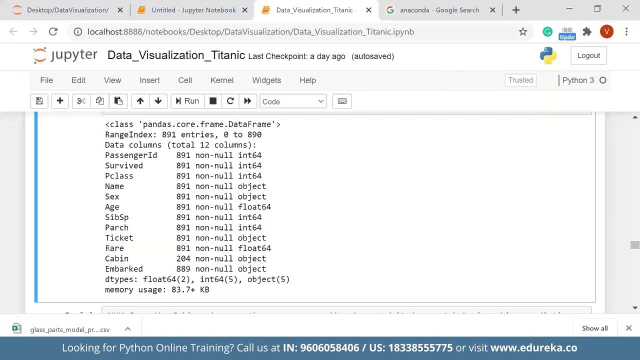 OK, all others will help you. FAIR will help you to figure out that person is a rich person or not. generally, rich people go into the first class and second uh, and all those ticket price will tell you that person's status. all others will have some. 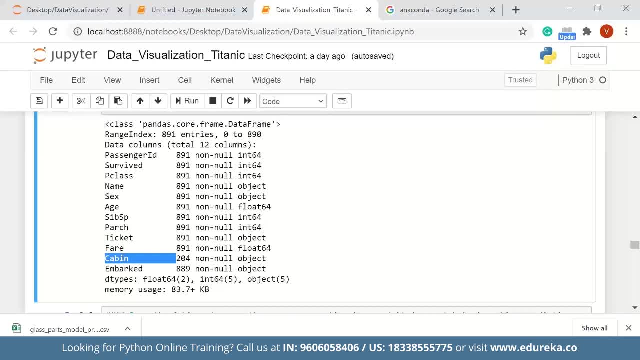 information but cabin you may not have much information and you don't have much data also, and not many people are allocated cabins because there are only two cabins. so in those rare circumstances you can delete that, saying that, okay, i don't need this data. okay, so then you are certain that it is not useful for this one? then we can delete that. 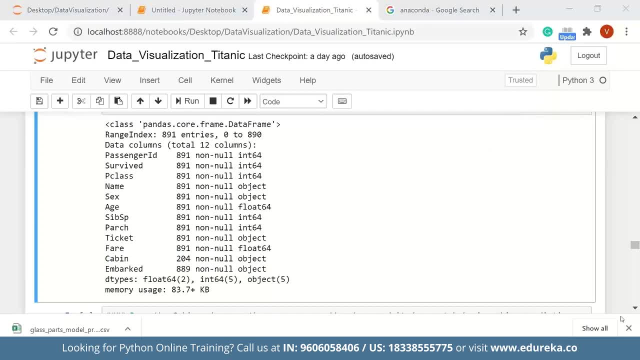 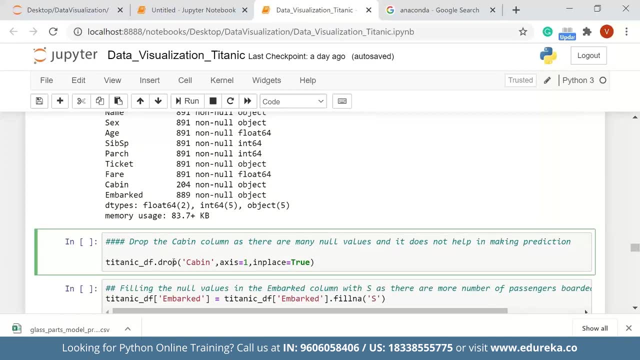 how to delete that, let us see. so, cabin, we assume that it is not useful, so let us delete. so the delete is basically drop. if you say drop, cabin, okay, access means row wise in place, means permanently delete. if you say false, it will delete temporarily later if you. 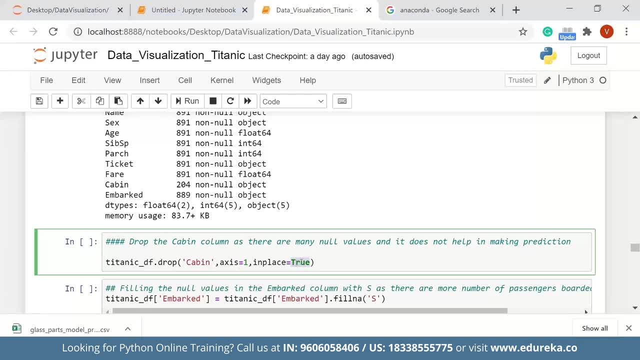 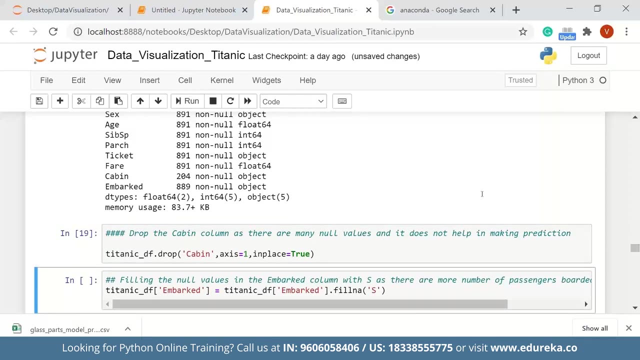 access it, you can get it, but we are saying that permanently. delete it. say true on all the rows where there is cabin. so if you execute this one, it will remove that cabin data altogether permanently. okay, let us delete that. we don't need that data, so we delete it now, if you see. 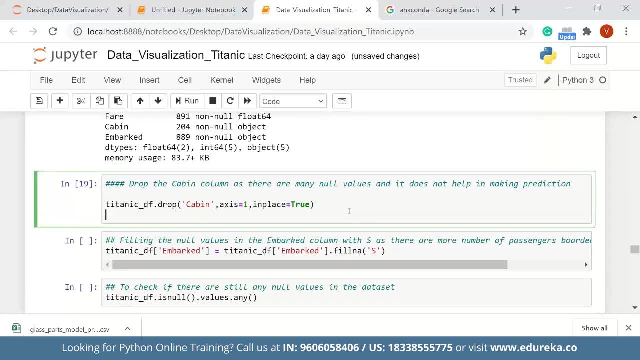 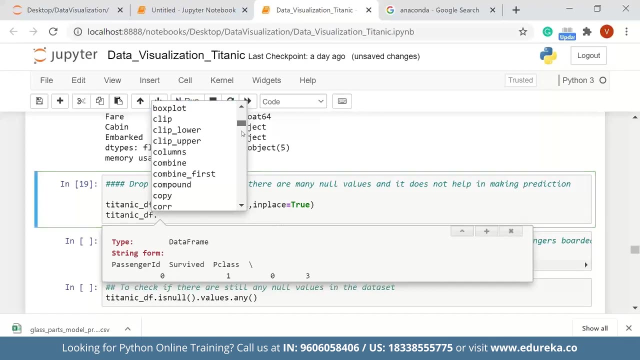 that the cabin is gone. okay, if you want to make sure, you can say that: titanic dot info. if you don't know the functions, basically, if you press this it will tell you. if you press a shift and tab, it will tell you all the methods that are associated with that. you don't need to memorize. 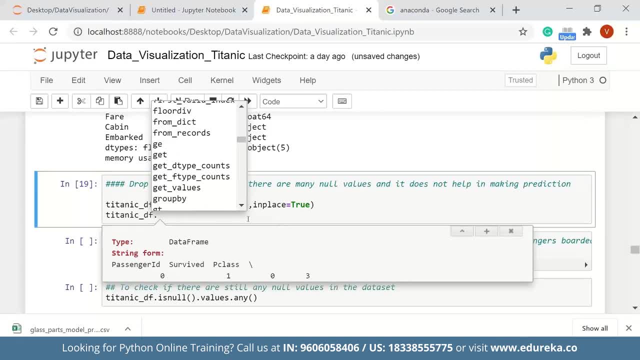 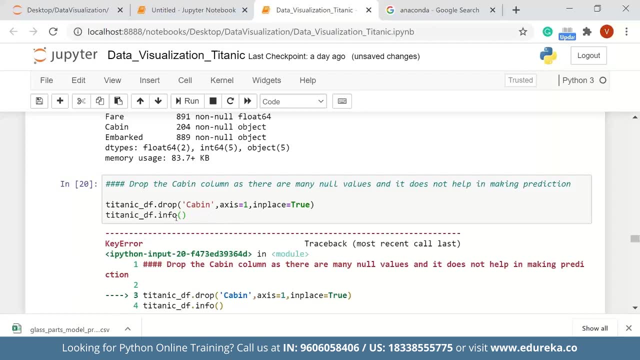 this. but as you use, you will get most of the method memorized. so if you say info, it will get all those things right, or describe you. you can say describe, describe, you will get that. whatever the data we are looking at. we are looking at the data. we are looking at the data we are looking at. 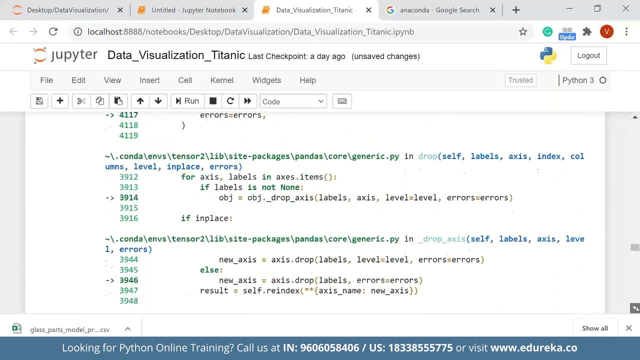 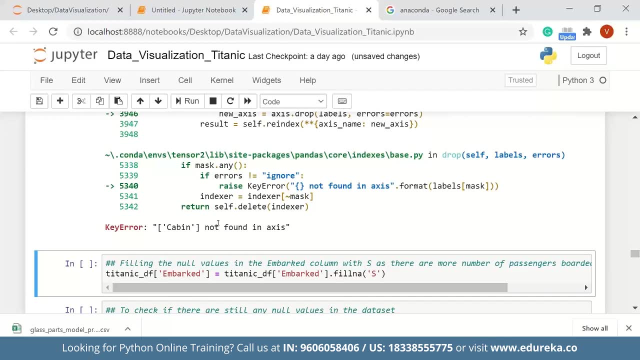 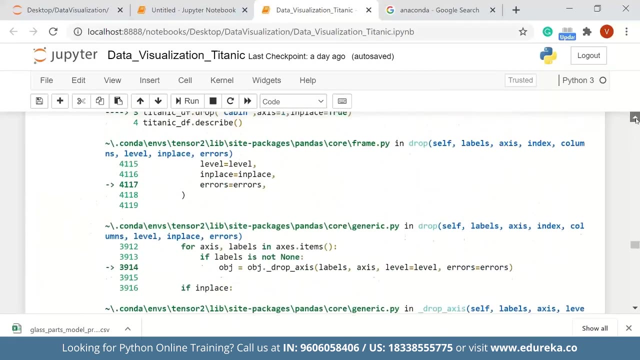 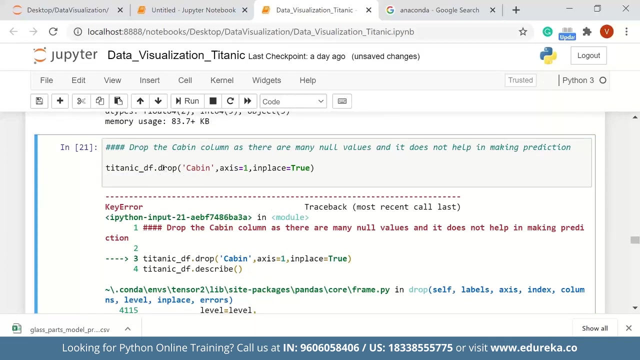 what the error is. okay, cabin, it is basically we already deleted, so it is giving error, basically. so let us put that in a different cell so you won't get there. okay, let me go to that. so this one. it is already deleted, so it's not finding that. so how to do that? create a cell. 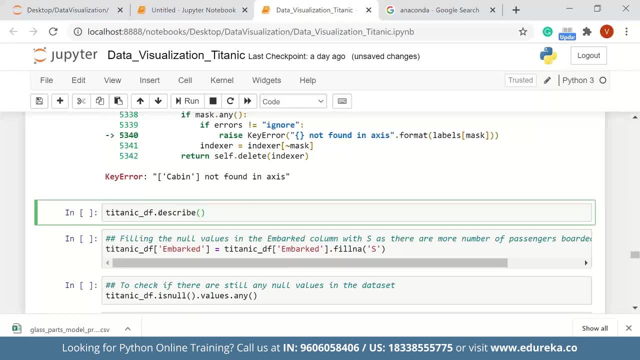 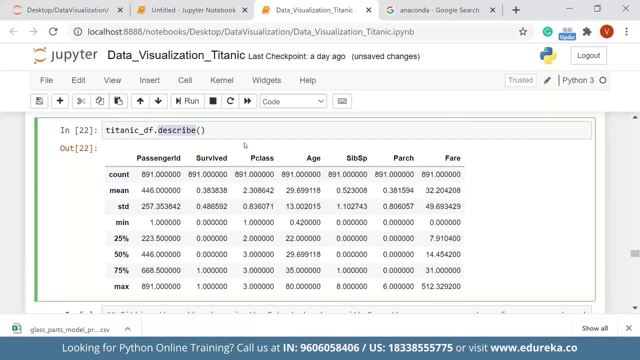 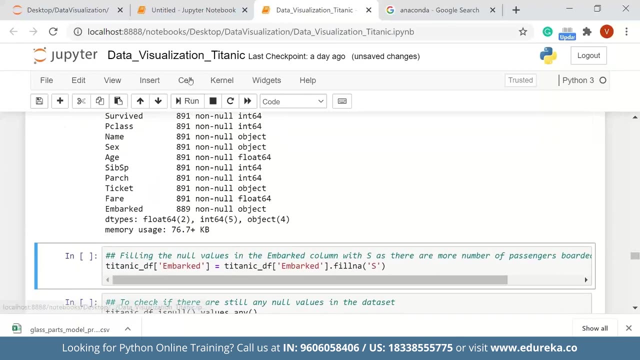 below and now do it here. so here we can see that cabin is gone. okay, if you say info also, you won't see that. so cabin is gone, we deleted that. okay, if you try to delete twice then it will give you error because it's already deleted permanently. now mbox: okay, mbox also has two records missing. 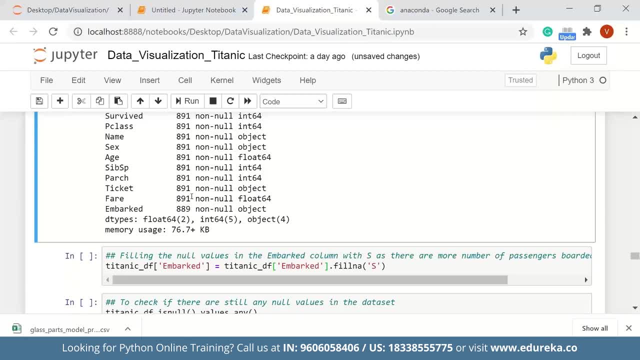 right, you see that 889 and the 891 are the total, so there are two values missing for mbox. so you can say that, okay, let us fill that one with the most frequent one, which is s. here we can use mode or we can fill with what. 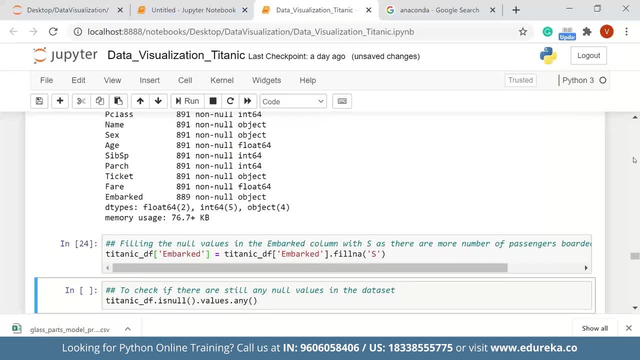 is the most common one in the data. this is where we are using that okay mode is the most common one. okay, so southampton, here is the most common one. so here, these are all methods that we are using because these are associated with this one right, these are associated with an object. so if i say here: 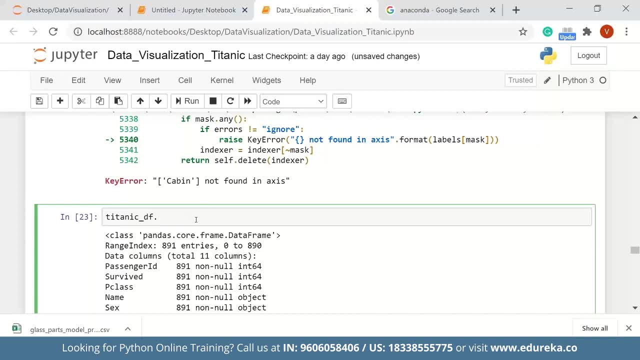 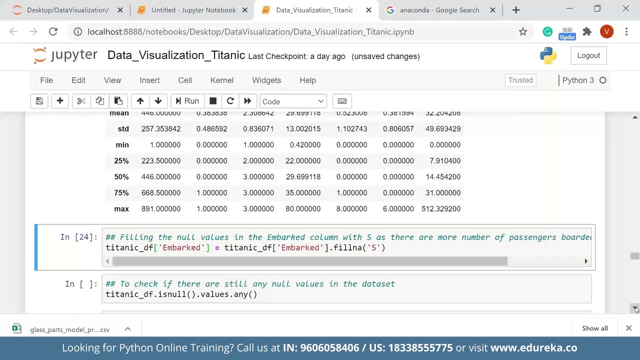 this info. info is a method, so all those methods, what you have, you can see it here, okay, all those things even describe is a method here, okay. so attribute means it will give some information about that object. method means it will do some processing, basically it will implement some logic. okay, the 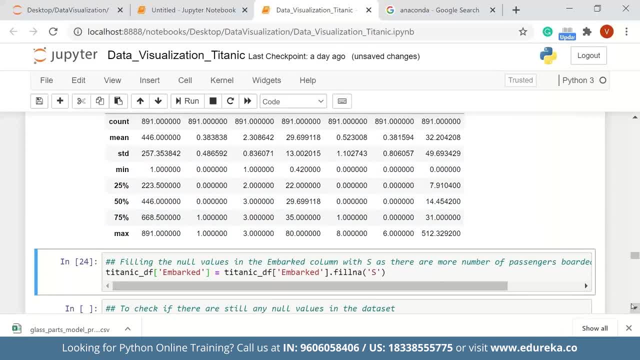 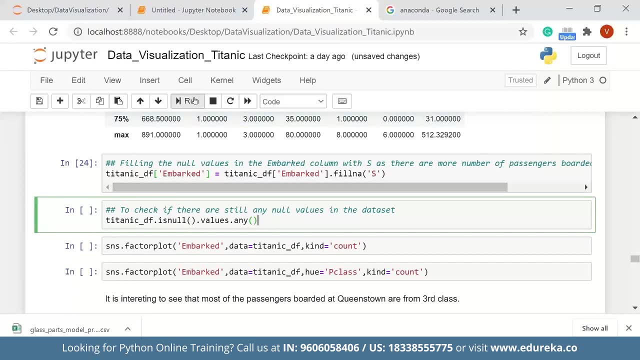 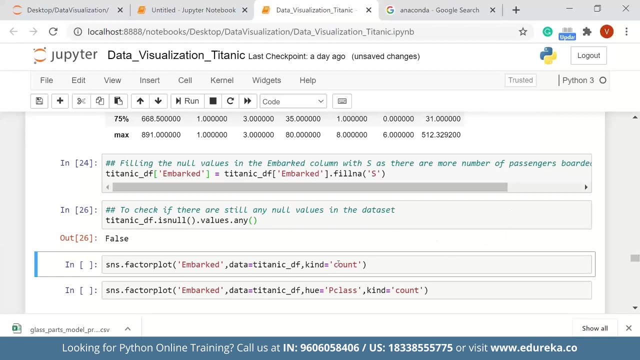 description. it is calculating all the stats about this and giving it to us. okay, so let us go further and see that. now we want to see: are there any missing values in the data? let us see that. okay, we filled all the missing values. now there are no missing values in the data. okay, then let us go and 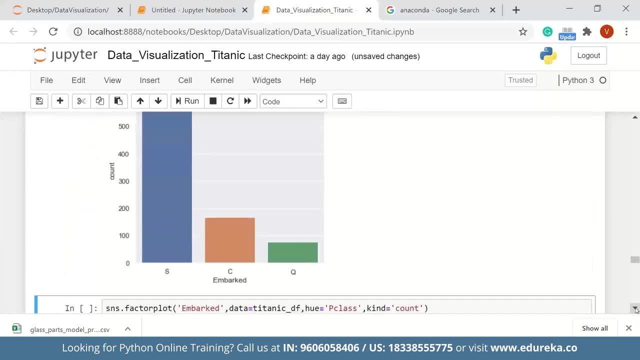 analyze the data and look at the predictions, basically, okay, so mbox, basically we want to see who embarked at what place. so, southampton: most of the passengers get on the ship and then there are few people in cork and queensland. okay, so the other thing, we will. 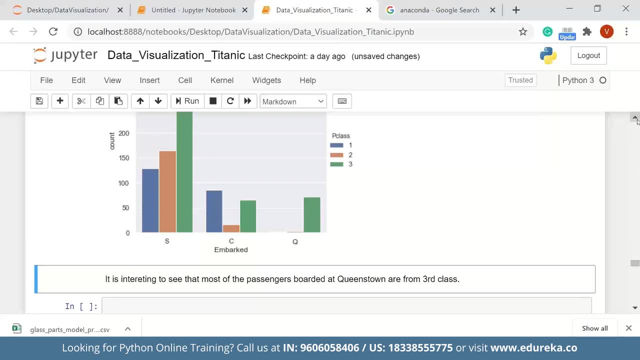 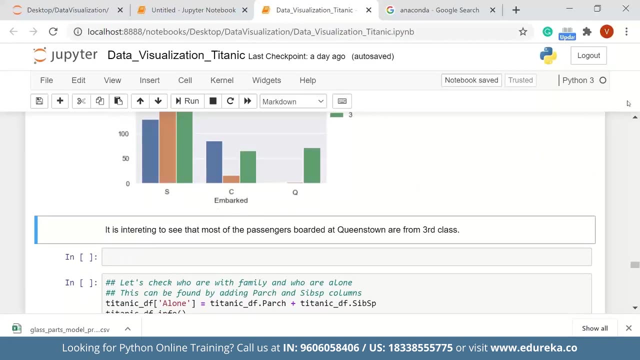 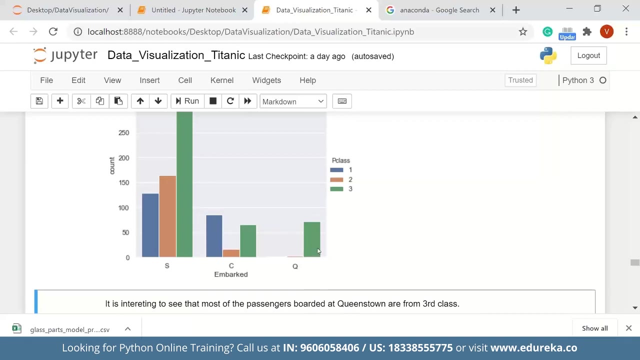 generally look at is basically if the data is balanced or not. so these are all the things that we will see to see that what kind of data we have. okay, what kind of data we have. see if you see that passengers at the queenstown this queue who got on that one, almost all are on third class. there is only couple of people in the second and 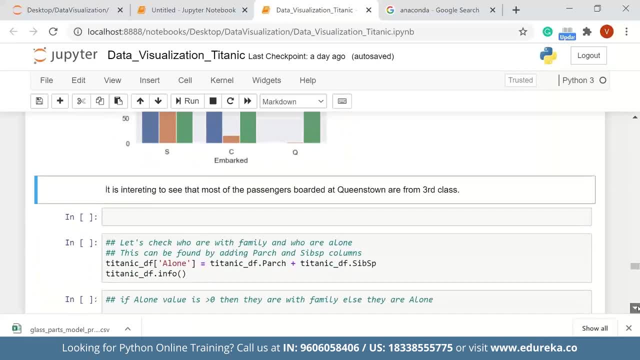 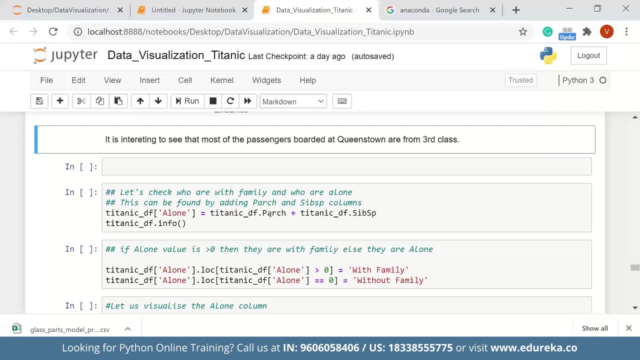 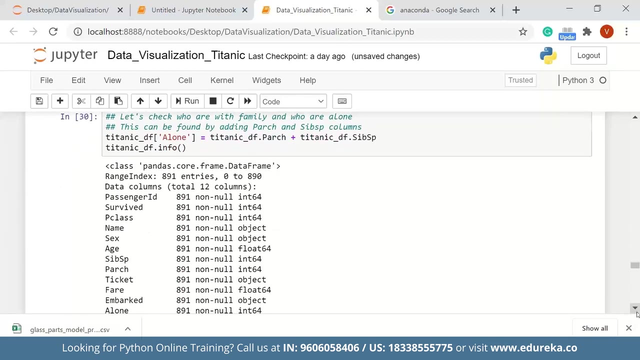 there is nobody in the first class. so that kind of insights you can get into this one. now we want to see that. okay, who is alone traveling alone on this ship? that means we want to find out whether people with the family are alone. so here we are creating features here this alone is. 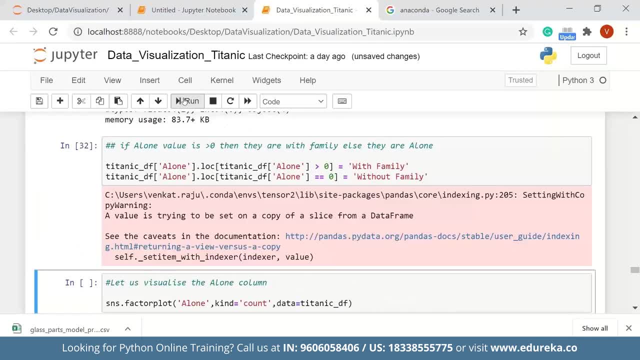 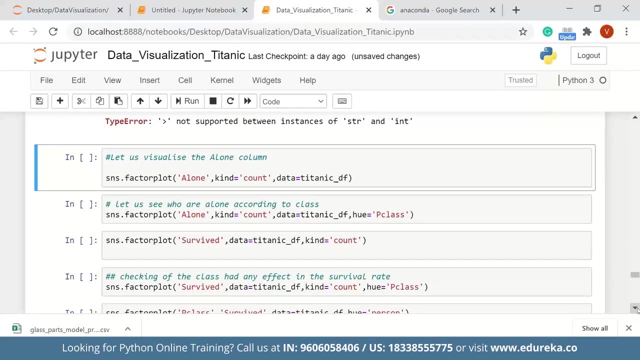 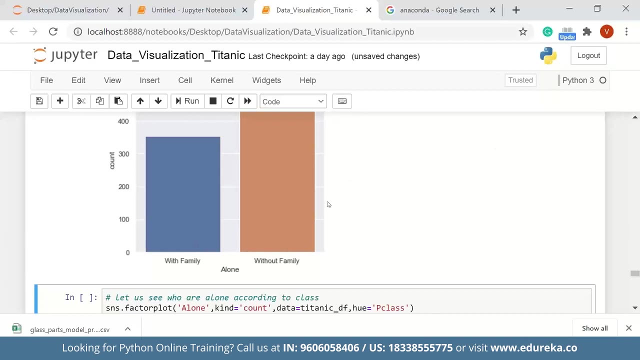 we created this one. why we created? we want to analyze that data. who is going with the this one and who is going without that? okay, so we'll see the other one. how to plot this. who is alone? okay. who is going with the family? you see that most of them are alone, not with the family. okay then. 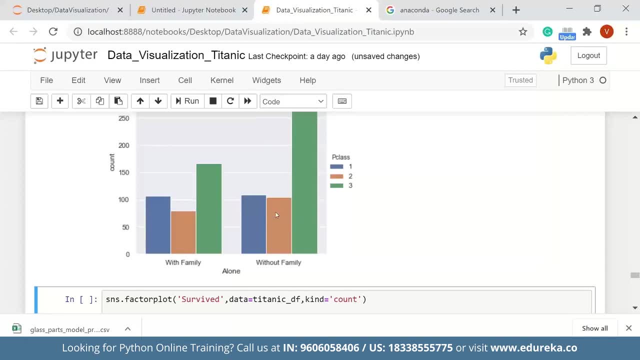 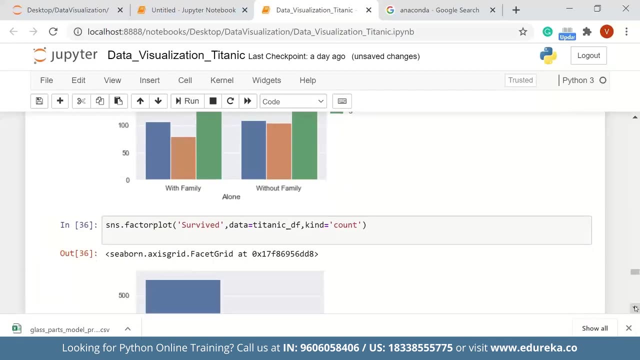 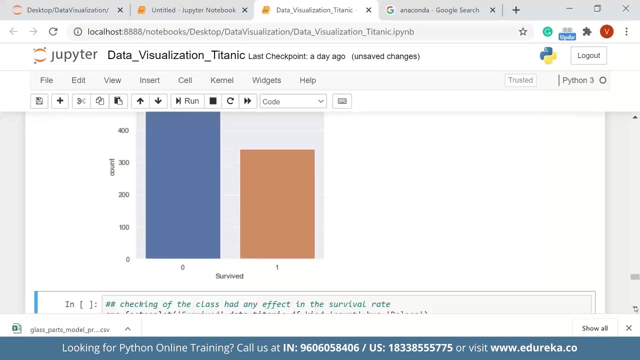 who is in the class wise, who is with family and without family. okay, then we'll see that who is survived and who is perished in the text. okay, so many people did not survive and few people survived, and this is the data for them. one means they lived, zero means they. 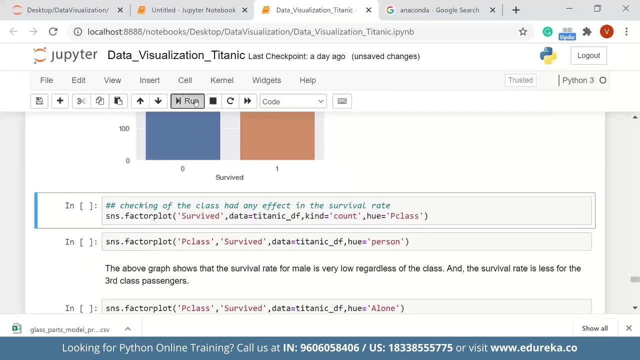 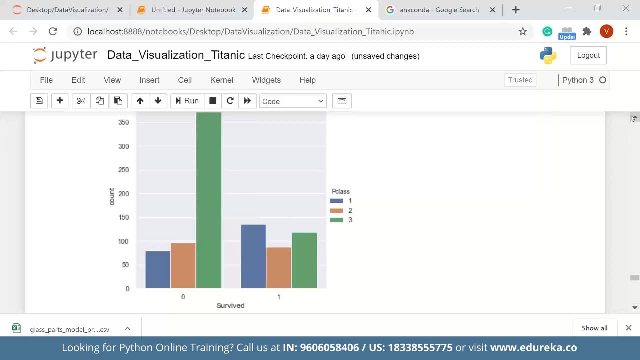 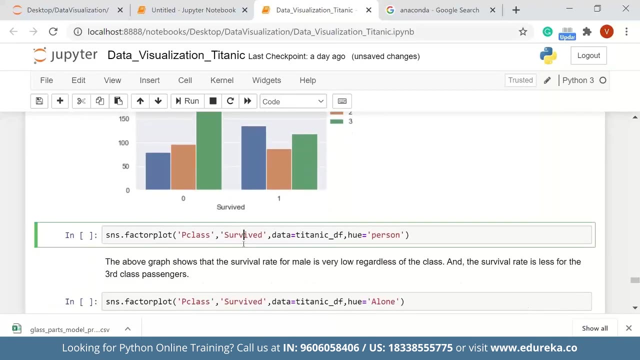 died the person they died. okay, so let us look at that and see that. what kind of survival is there in each of the class? okay, so this is the kind of analysis that you need to do for all the people, all the passengers and all those things here. okay, 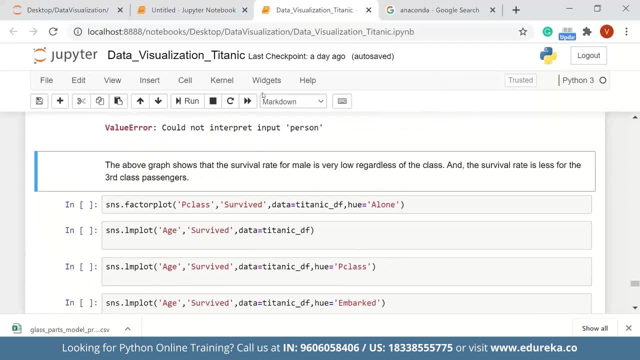 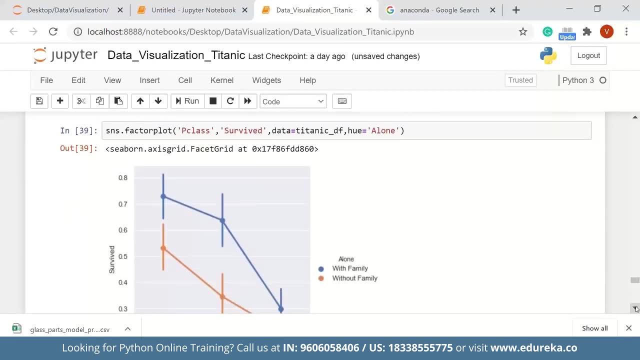 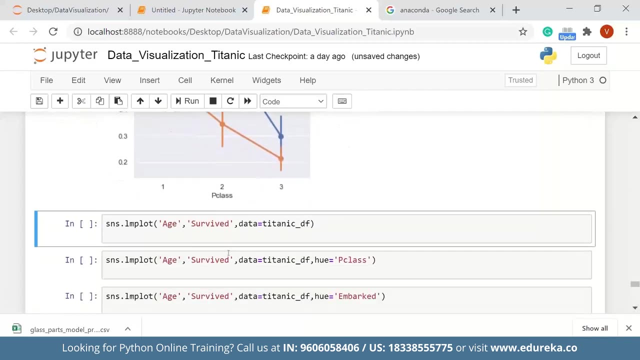 we have to create a data item called person and all those things, and you can do to do or analyze all those things, okay, and then you can plot these plots where you can see the distribution, who is with family, without family, all the distributions you can see here, okay, 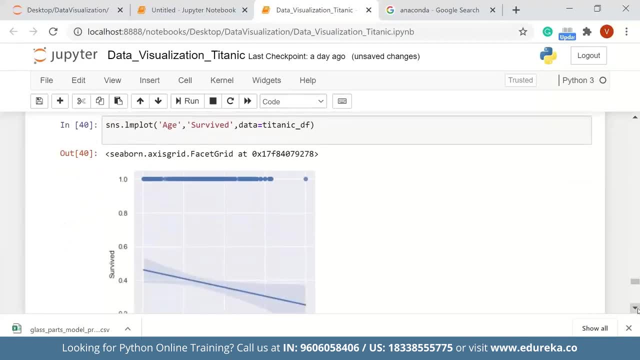 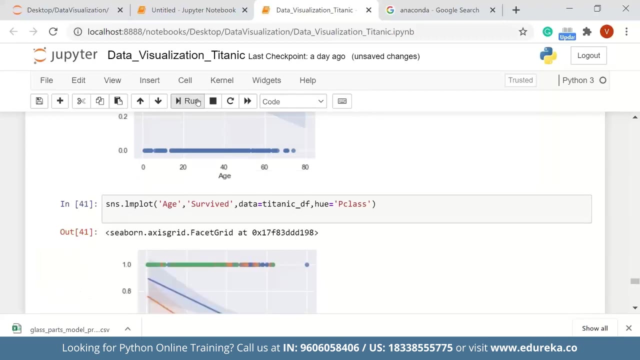 age, with the distribution, with the age and how people survived, people died, and with the age. basically is the survival rate is moving with the age. now you can see that it is okay. so let me quickly go through these so that, by class, you can see the survival and then 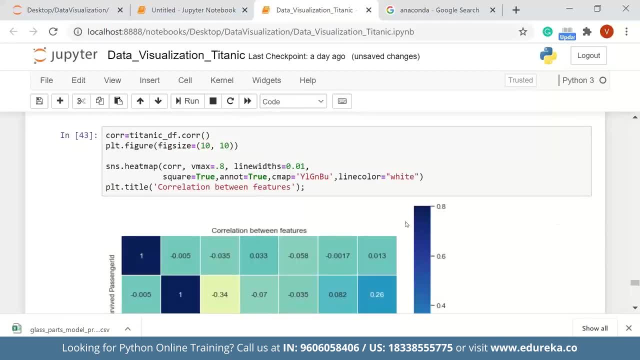 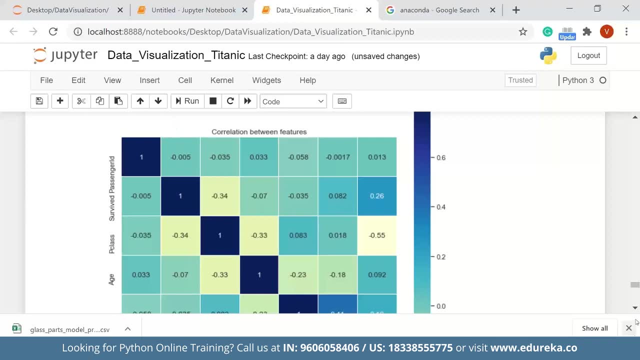 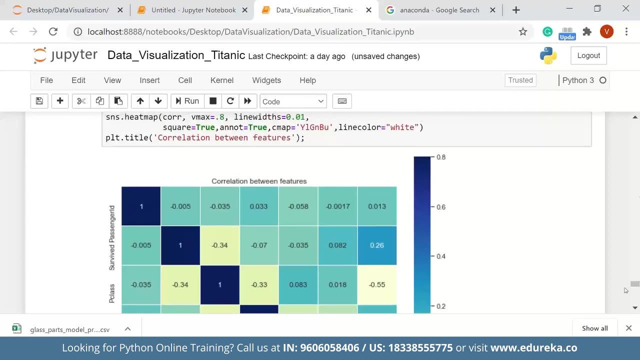 by age, all this kind of plots you can do, then you can construct something called a heat map. that means: what is the relationship between all these things? so here this is called p a heat map. here it is between one and minus one. you can see that it is between one and minus one if it is. 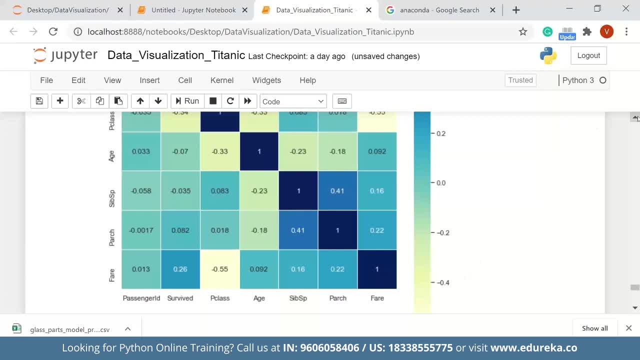 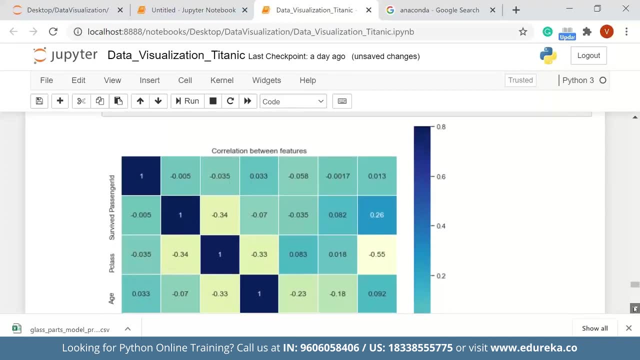 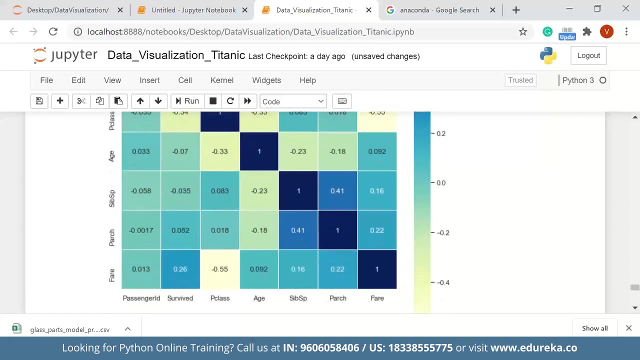 minus one close to okay, that means it is inversely related. if it is close to positive one, that means it is directly related. so you can see that this one means directly related. okay, let us see that age is directly related to age. only here also age, so age is directly related, so we ignore this. 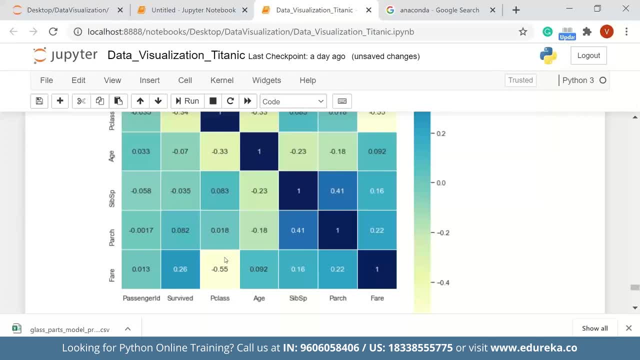 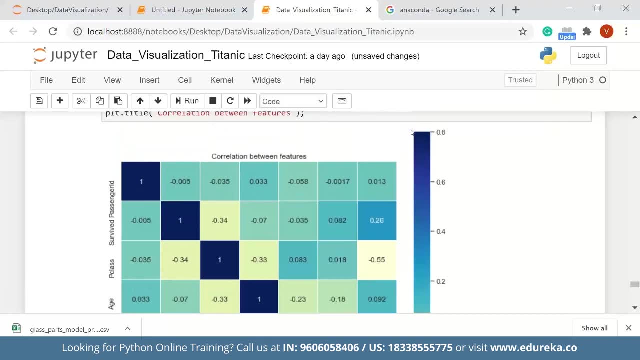 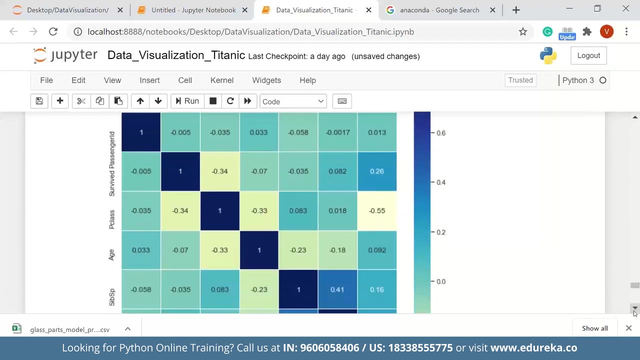 diagonal and ignoring the diagonal, because each is with its own. obviously it is. age is highly related with age. other things we can look at this one. so what is the highest here? so let can anybody see that what is the highest correlation here? that means, what is the? 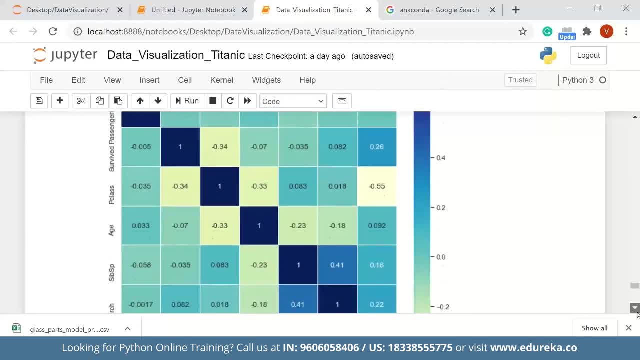 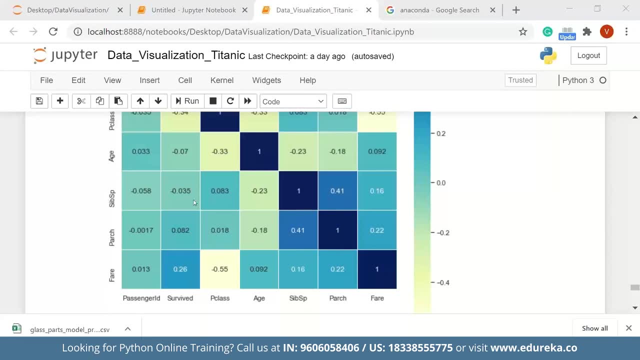 highest number among these. you can see the color coding and see the. what is the highest one? you see here the parent-child relationship and siblings force. obviously, because the person has brothers or sisters or wife and husband generally, it is probable that they will have kids also. so that is what this relationship is saying. 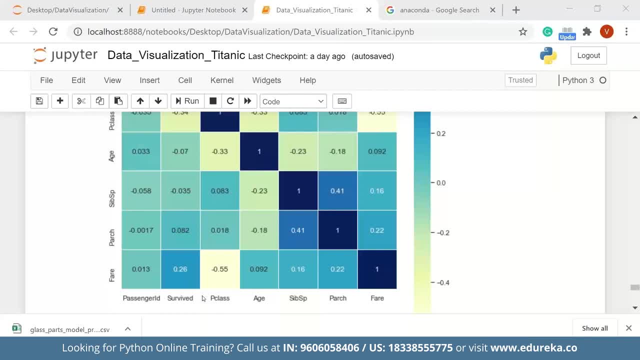 then that is what this relationship is saying. then there is something survived and fair. this is also a little bit correlated. that means if the person is rich, more probable that that person survived. okay, so these are all the things that you need to look in a heat map. okay, so let us quickly go through the other kind of things, okay? 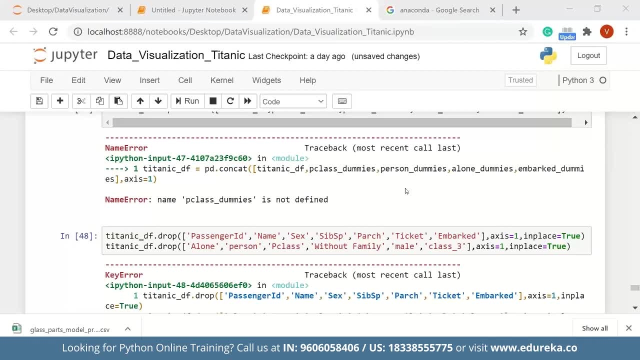 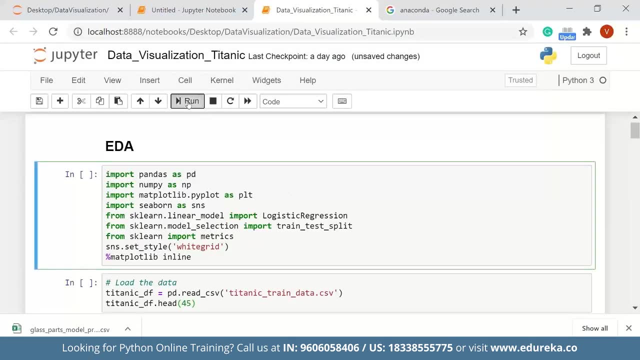 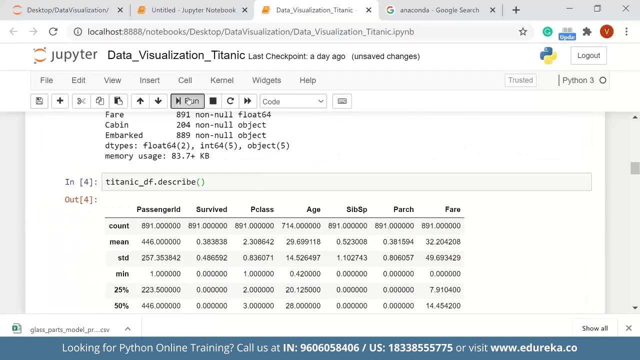 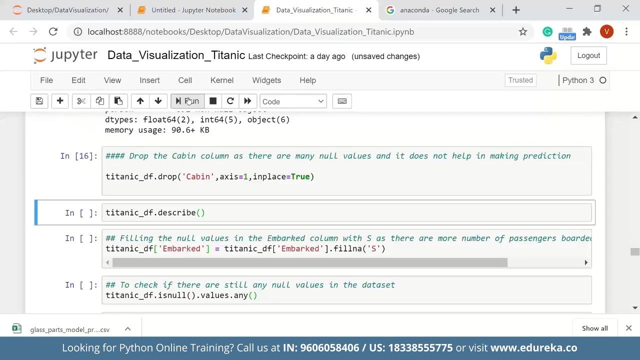 let us quickly go through that. so basically, sometimes if you mess up the kernel, you can restart. there are other ways of doing this. that means you can execute the entire file at one time, okay? so basically you can execute these things in the order, okay, so you don't miss anything. 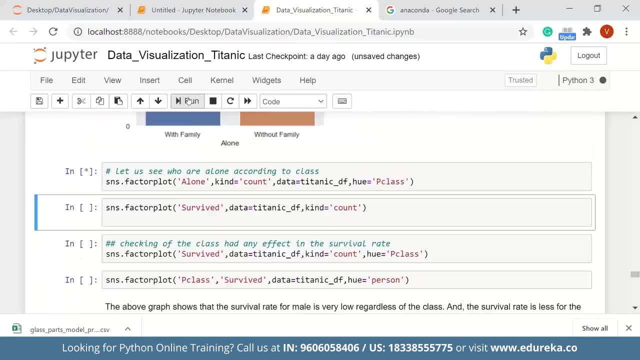 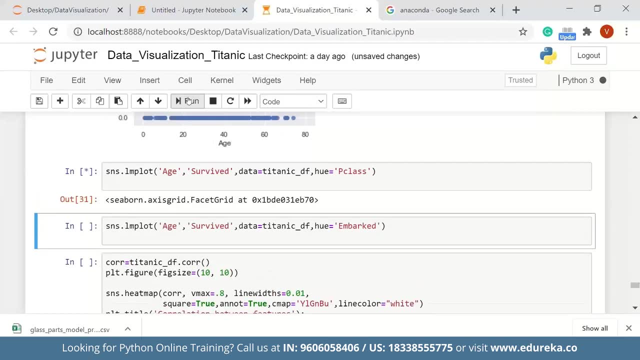 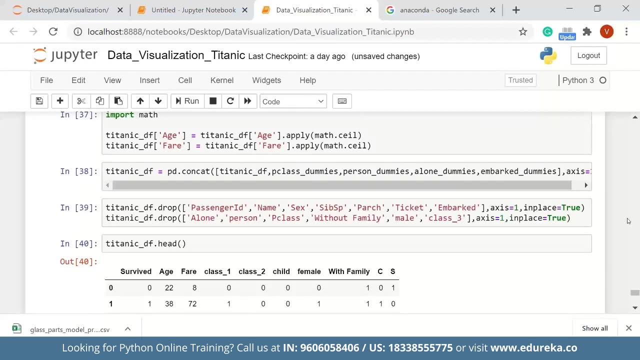 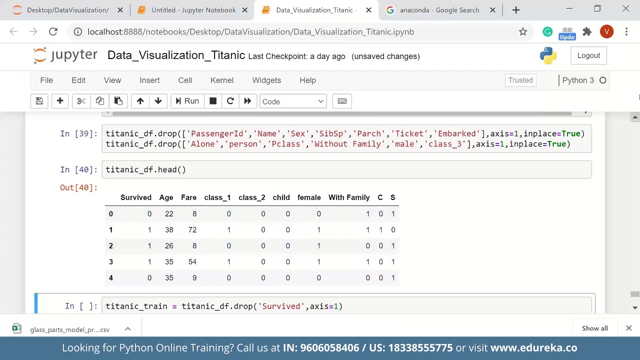 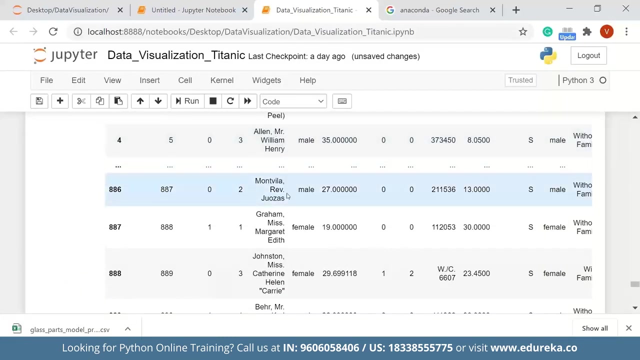 and then save this one basically, okay, okay. so basically, once you execute, we convert all this data into the numbers. that's what this one is doing. basically, what we are doing here is get the miss means here. these algorithms need only numerical data. any data that you have in the text format, computer can't understand that, so see name. 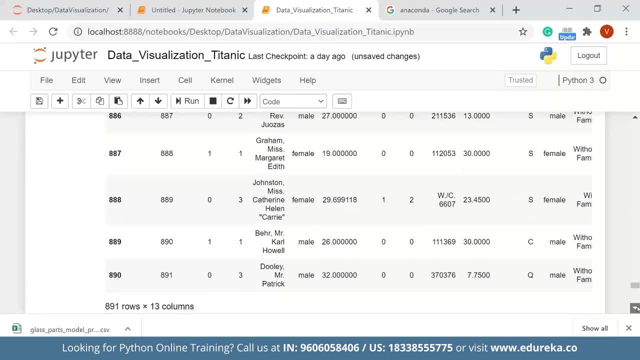 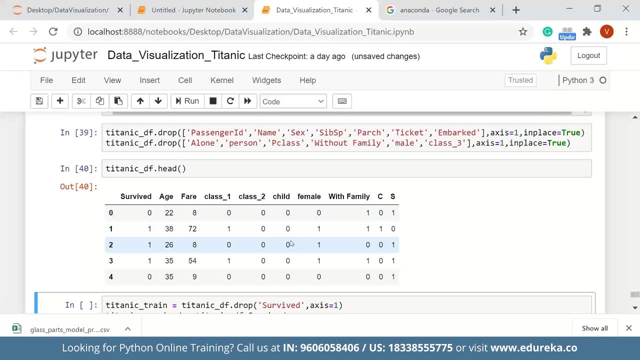 or male, female. computer doesn't know what is male, female, so we need to convert into the numbers. basically, it will do all kinds of mathematics on this one. it will do lot of transformations, high level matrix multiplications and all those things it will do, but in that it needs numbers. okay, that's how the machine learning will work: only on numbers. 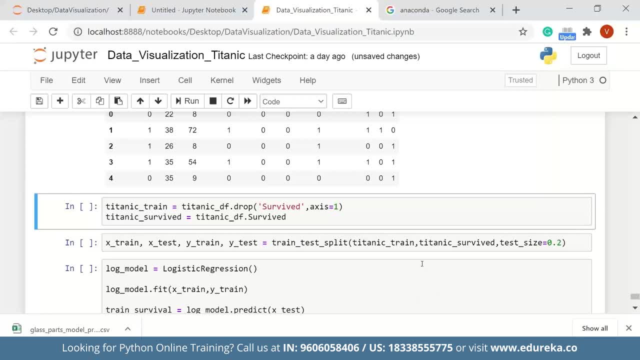 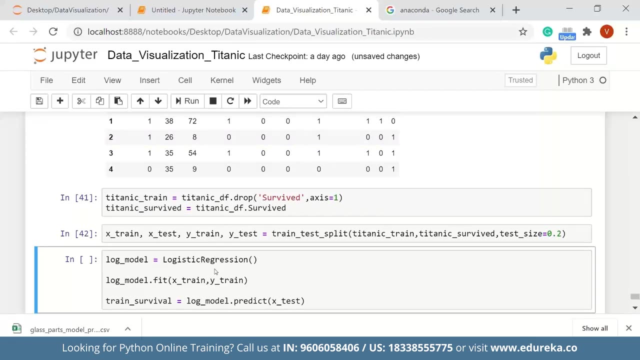 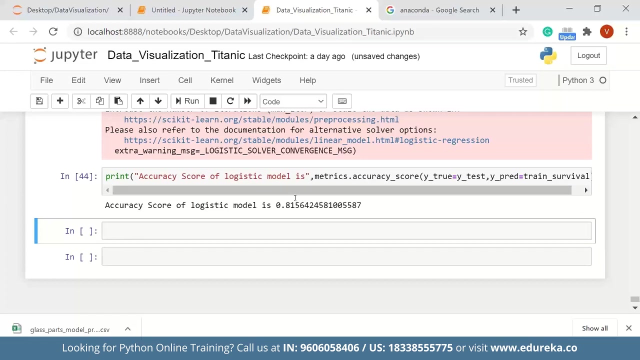 artificial intelligence. it is everything about numbers. even when you want to show image or video, you have to convert it into numbers. that's the point you need to remember, okay. okay, then what we do is put this data into training and testing data and use a model to predict the survival. okay, so that's what it is basically. once you predict. okay, now you have. 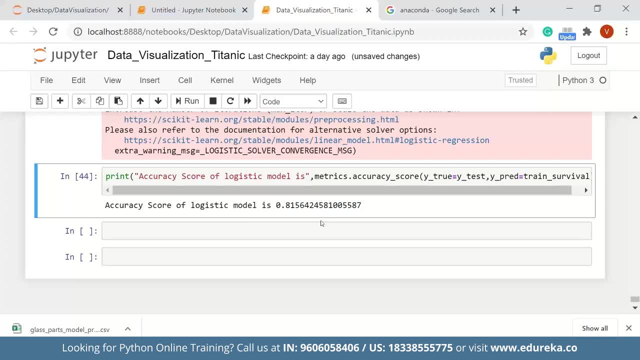 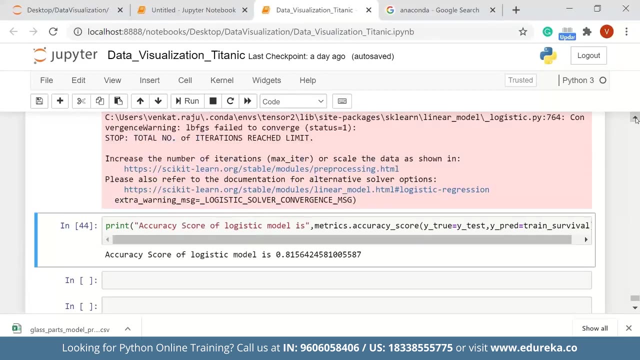 this much accuracy: 81 percent accuracy. that means your predictions are 81 percent correct. 81 times out of 100 it is correct. so this is basically a model building. so here we built a machine learning model using logistic regression algorithm. we built an algorithm here. okay, so logistic regression is. 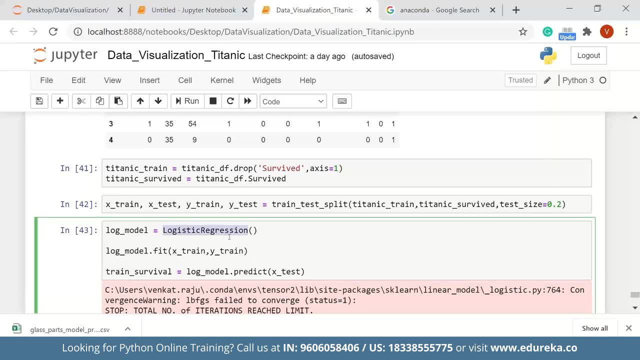 what we used. there are 40- 50 algorithms like that. some of the most popular ones are linear regression, logistic regression, svm, support vector machines- okay, xg boost. these are all the popular ones. you can use any of them. there are two ways of doing it for classification. 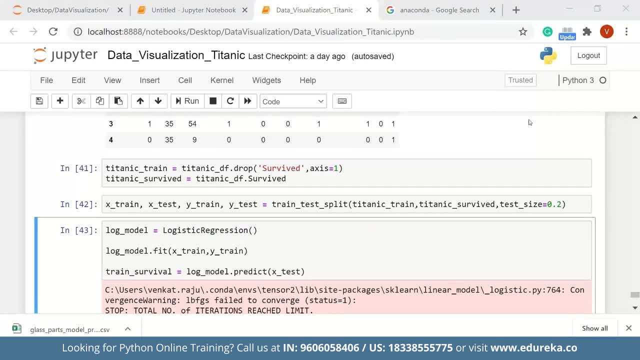 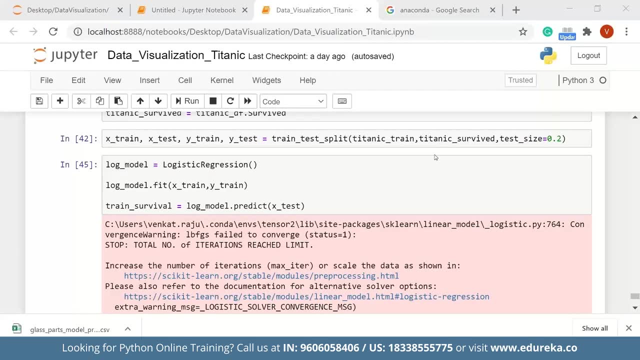 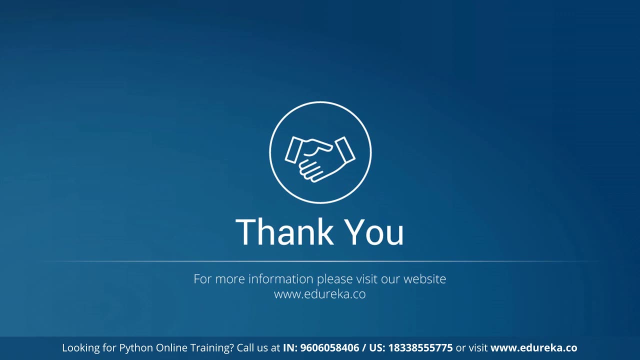 there are some algorithms. regression, there are some algorithms. so that is what the machine learning is, what, eda, we need to do. okay, thanks a lot. we hope to see you again. okay, thank you, you, you.